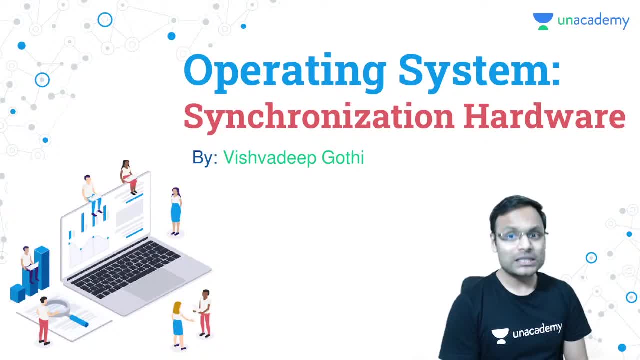 So what are the hardware solution and why we call those solutions as hardware solution? We will definitely talk about it In this particular session. So, without any delay, let's get started. Before we start, let me introduce myself for those members who don't know about me. 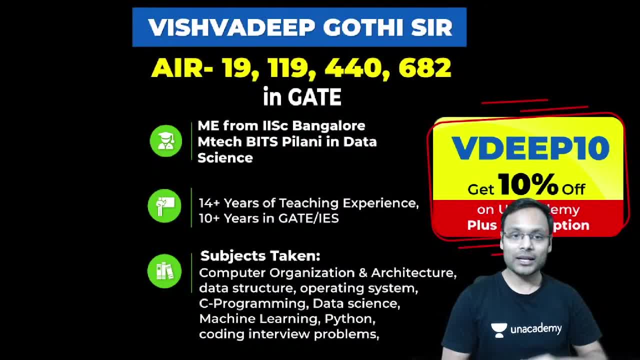 My name is Vishwadeep and I am working as a channel leader on this particular channel. This is my profile. If you are having a will of learning, this channel is having so many pre-recorded plus so many live sessions for you and your learning. 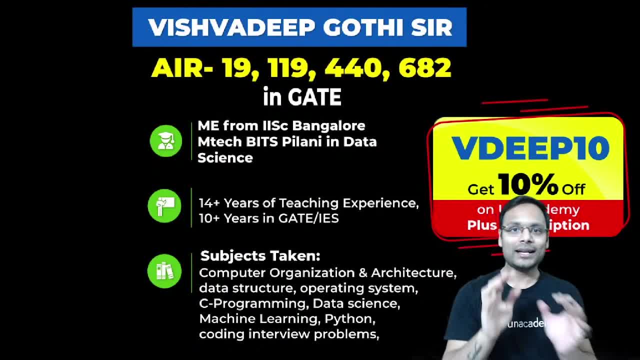 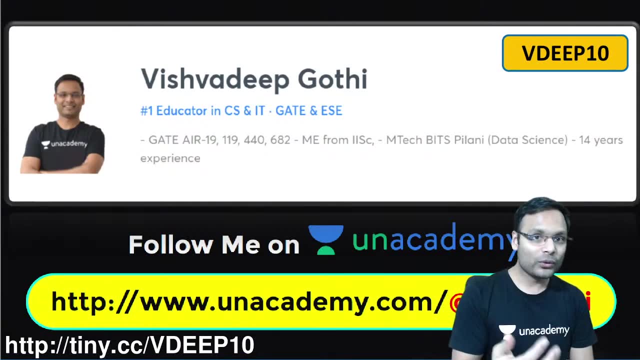 Utilize it And I will make sure that entire channel will always work hard, hard work and dedicatedly, always work for your learning. If you want to learn more in more interaction, like you, want to share your problems and your queries, your questions, with the image form, then you can log on to Unacademy and you can utilize its facility. 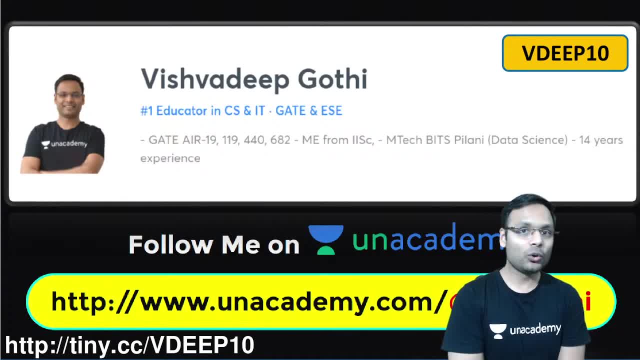 Unacademycom page out, or you just download Unacademy learner app and follow my process. Once you follow my profile, you will be able to access my special classes, which are recorded. plus, you will be able to learn from my live special classes. 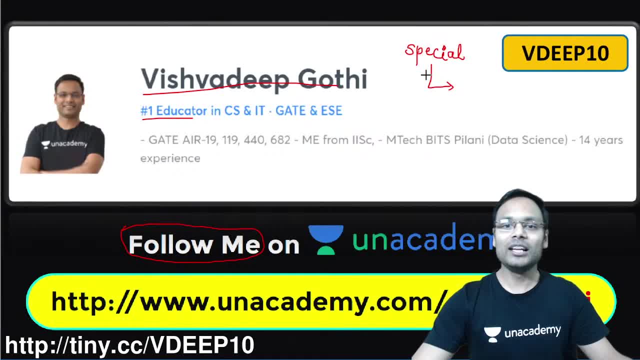 Also, once go through it, you will definitely learn a lot. Unacademy provides you lots of content free, including practice questions, special classes, including the quizzes, test and the lots of lots of content. So this Particular content you can unlock for the very first time using this code. 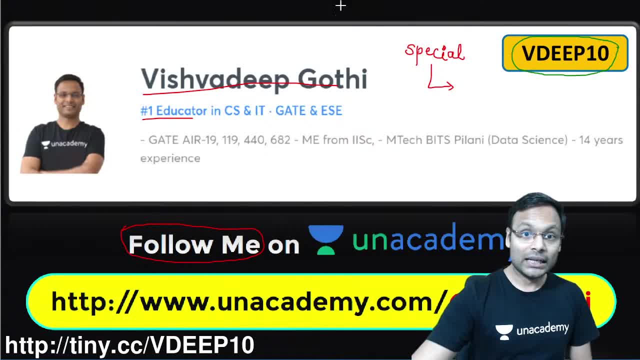 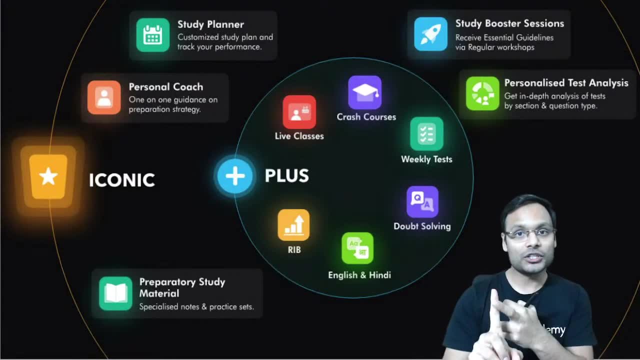 We did that. if you are preparing for it and you are feeling like you can do every single thing by yourself, your thoughts are really great. Keep going in your profession with more structured preparation plan, with more structured and organized and efficient preparation, And you should utilize your time in such a way that you don't waste much time. 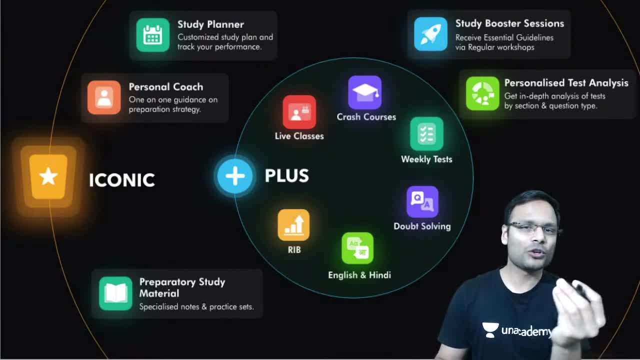 In just finding the solution of a question, or finding the solution of a small doubt, or finding for the content which content to follow and what not to do. If you are doing this kind of time waste and if you want that you want to utilize your time to the perfection. 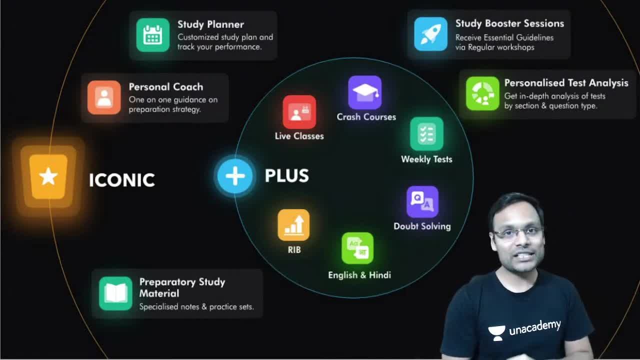 If you want to go for such a preparation, which makes your preparation more efficient in terms of whatever the amount of time you give for the preparation, it will be paying off to the same amount- Then go for an academy plus subscription. This plus subscription will give you live classes which are interactive. 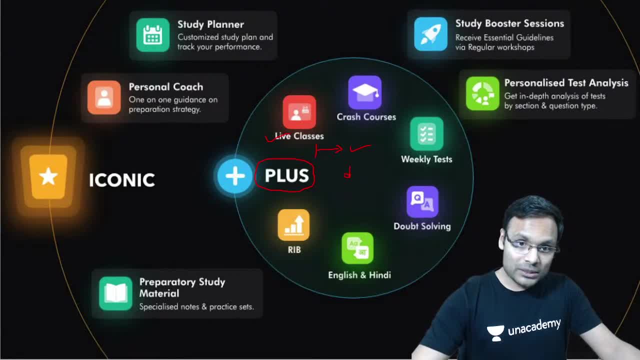 Hence your learning will be long. lasting. very important: in the plus subscription You will be getting daily practice questions so that you will have the learning how to solve the question using the given concept, Doubt solving weekly test, crash courses, guidance of an educator in the English batches and multiple such kind of things which are more important for your preparation, so that you can have the preparation. 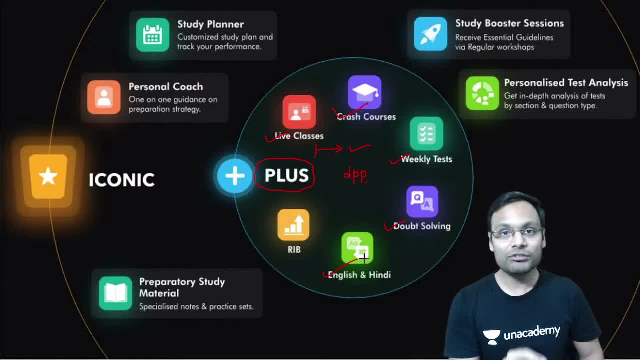 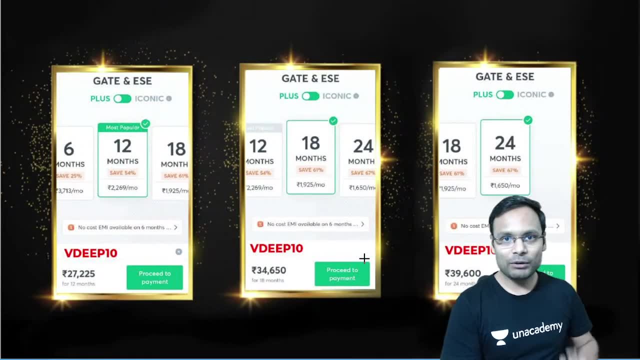 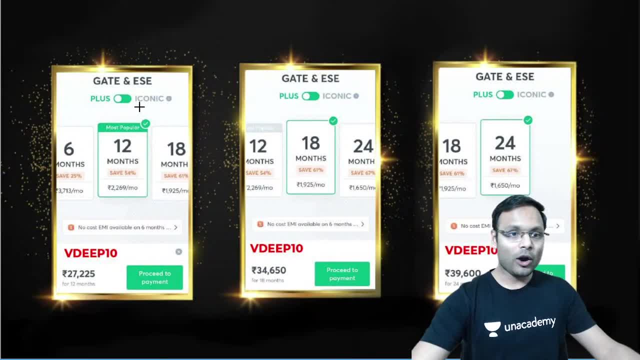 You can take subscription of any duration, Whatever you want, based on your preparation plan. Take the maximum duration plan so that you can utilize it and you will have to pay a less amount for per day or per month basis. Use this code in the time of checkout. 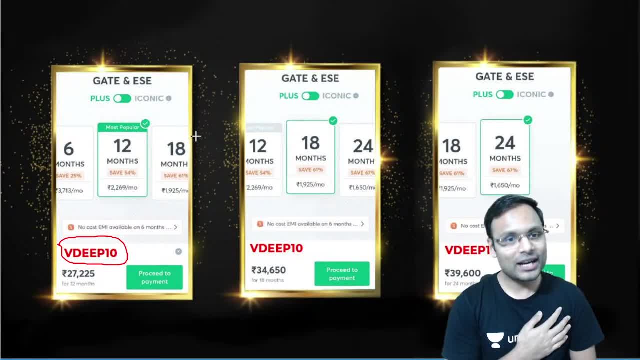 Use this code in the time of checkout so that you can utilize it and you will have to pay a less amount for per day or per month basis that you can get 10% discount, plus my personal guidance, plus my mentorship, if you want to study. 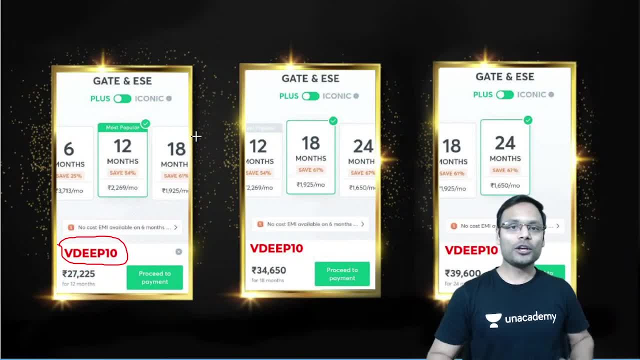 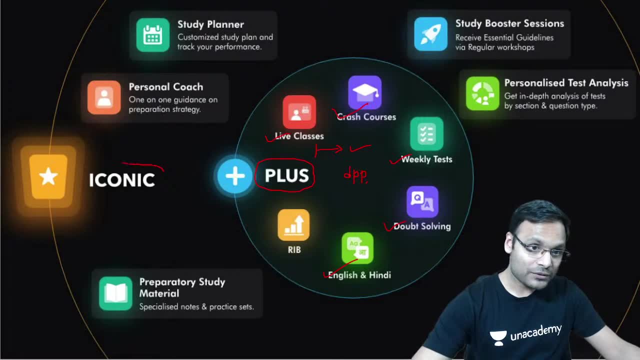 under my personal guidance, use this code and enjoy your subscription on an academy plus. if you want to take another type of subscription which is iconic, then you can go for it. this iconic subscription has all the benefit of an academy plus and another benefit of having a personal 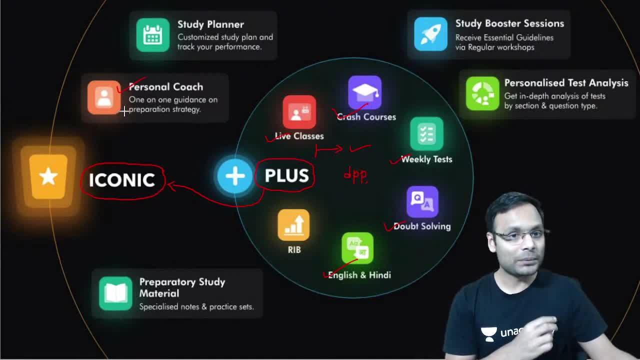 coach means you can go with more customized and personalized preparation. there will be an coach. that particular coach will give you preparation strategy. preparation plan will track your performance. will give you study booster session will give you personalized doubt solving will give you personalized test. analysis means whatever the problems you are. 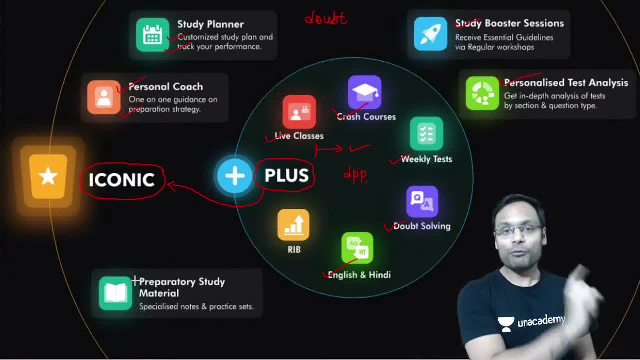 facing, there will be a person, there will be an expert, provided you from an academy, who will solve those problems for you, so that you will have only tension, only work of just preparing and preparing for the next step, preparing extra practice sets and notes. also, you will be getting in this iconic subscription this: 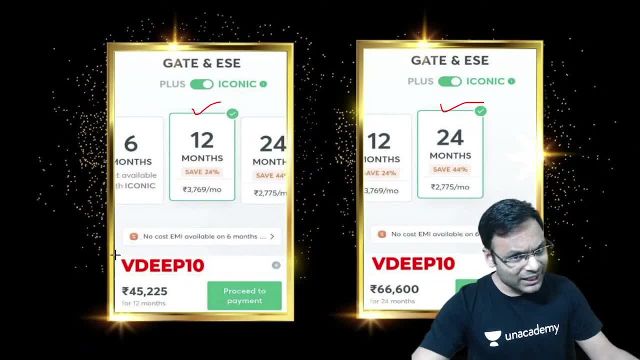 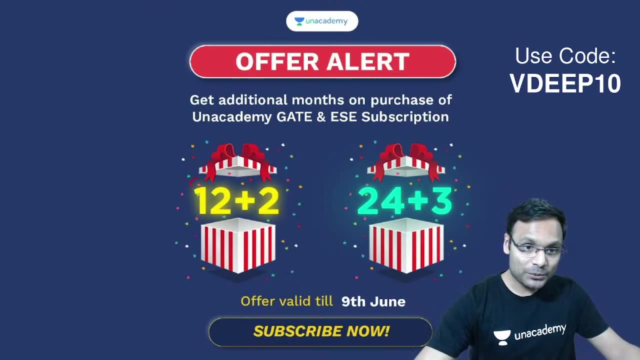 iconic subscription is available for 12 months and 24 months only and again, if you use this code, vdeep10, you can get 10% discount, plus my personal guidance, plus my entire team's support. till tonight we have a specific offer. offer is, if you take subscription of 12 months, 2 months extra. 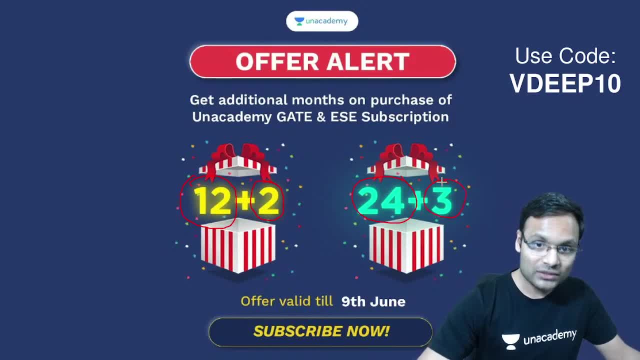 subscription you will be getting, and if you take subscription for 24 months, 3 months extra subscription you will be getting. So if you take this code, vdeep10, you will get 10% discount plus my personal guidance. plus my personal guidance, and this is only available till tonight. so if you take the subscription till, 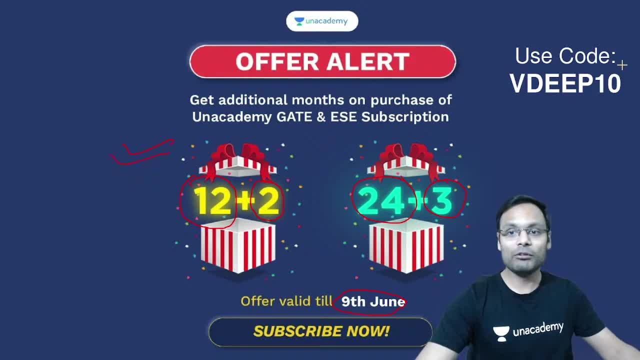 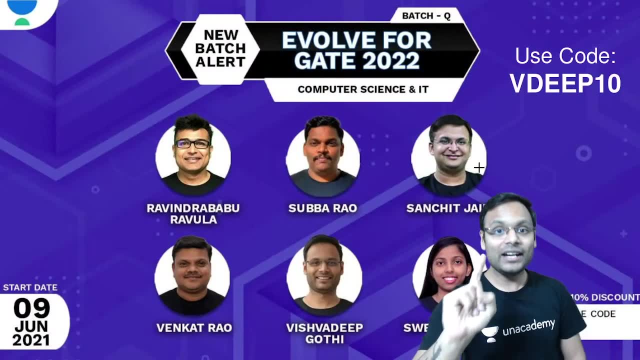 tonight, up to 9th June, only this particular offer will be working. use this code to unlock this particular offer in your subscription plan. and one more thing: ascend and evolve two batches we started. these batches were having your full length preparation up to gate 22. so if you want to join, 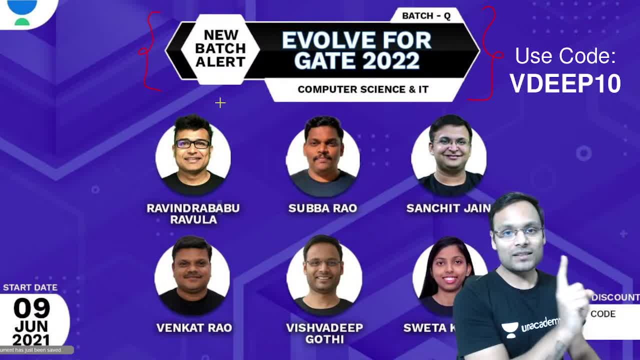 an academy plus. This is the last time we have starting a new match- evolved and ascend- for gate 22. after the, whatever batches will come, those will not be like evolve and ascend. so if you have the chance to take the subscription, take it now so that you can have your preparation comprehensively and complete. look at this: top educators of country are available on the platform who are ready to teach you in your best possible manner, plus my personal guidance. 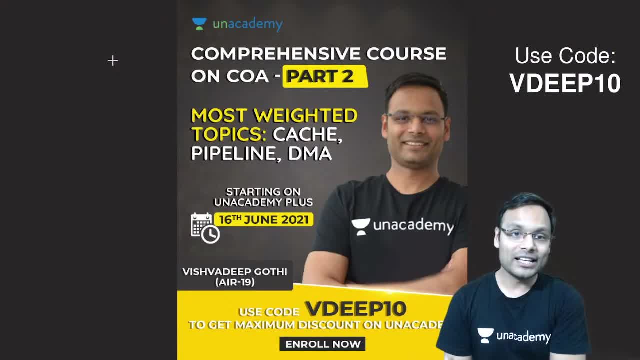 another second session is a starting. second session means the second part of coa is a starting, which is having the maximum wattage in the gate exam. every year one question comes from cash. every year one question comes from pipeline. this year one question came from dma, also very 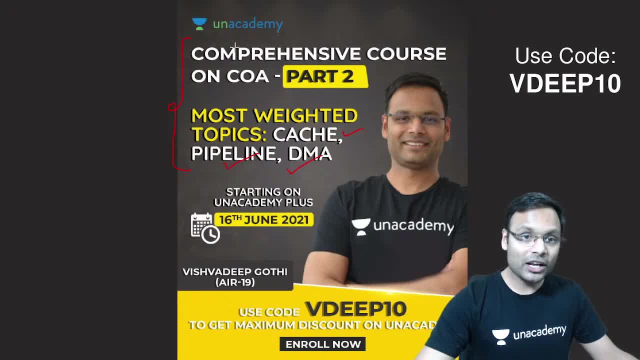 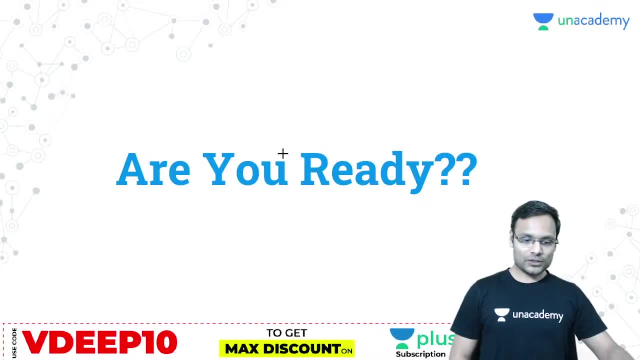 tough. if you want to join this particular comprehensive course which can make you feel like how to learn coa, then join the unacademy plus as soon as possible. but before i start the session, you all know that what exactly i need at this particular point of 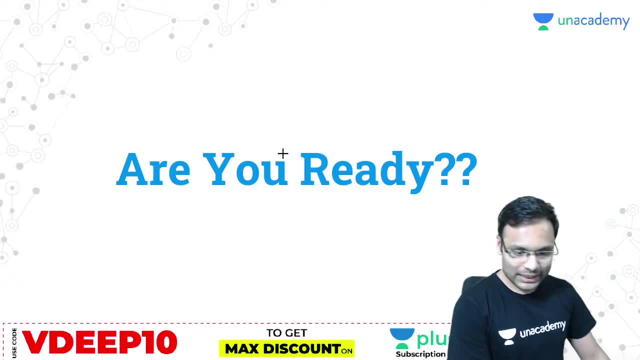 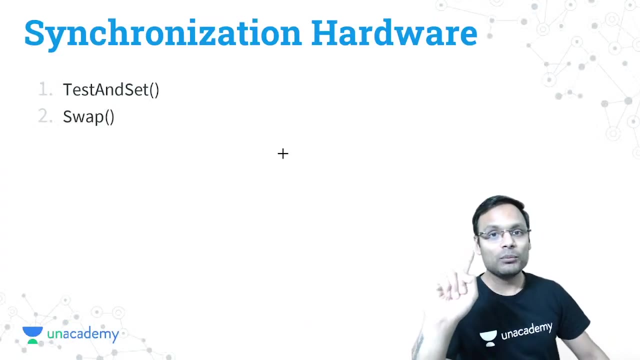 time. what exactly i will need from your end is your perfect concentration. all those members who are not able to learn live, i am asking you again: come live so that you can have more interactive learning and those learning will be more and more and more long lasting for you. 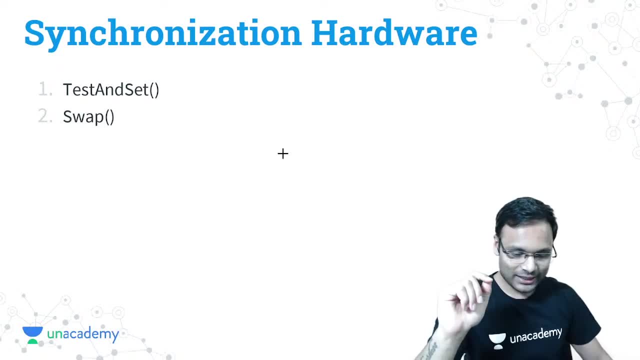 let's start the session. let's start the session. let us start the session. but before we start the session, this: what is the topic? till last class, what i taught you is how to solve the synchronization problem, or i should say critical section problem, using using what using the software solution means in the process code we will embed some kind of code. 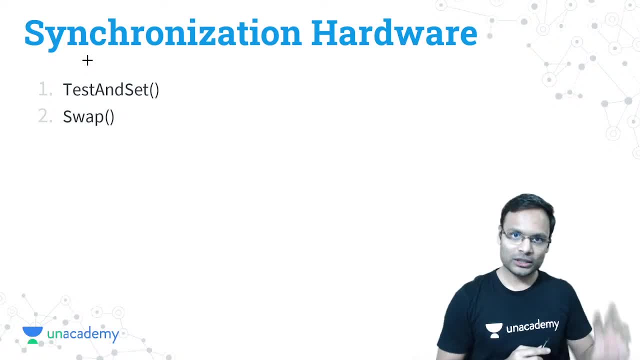 those code were providing the synchronization solution. three types of solution we have seen. one was log based solution not working properly. mutual exclusion was not there. why? just because lock variable itself was shared. then second solution: turn basis. it was giving the mutual exclusion, but progress was not there. why? 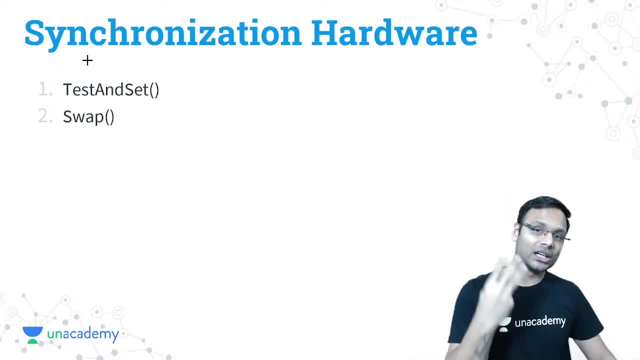 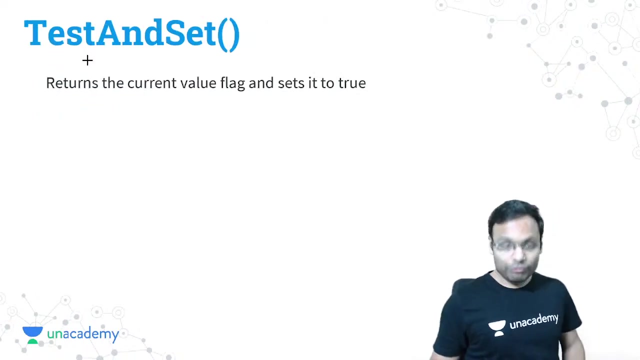 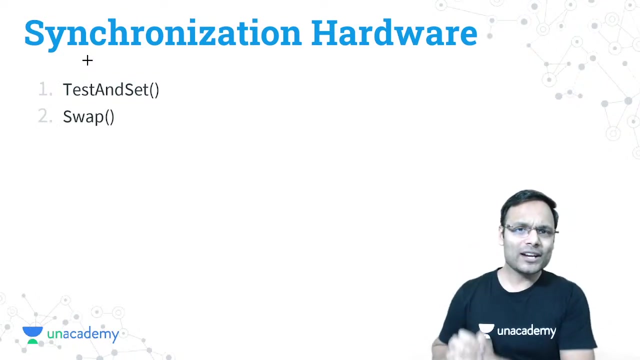 just because of strict alteration. then third solution: we have seen peterson solution. it was perfect. it was providing all three requirements satisfied, mutual exclusion also and progress also, and bounded waiting also. now, first thing we are going to discuss is now synchronization hardware. see, if suppose, if suppose we don't want our software solution to work, then a particular computer architect. 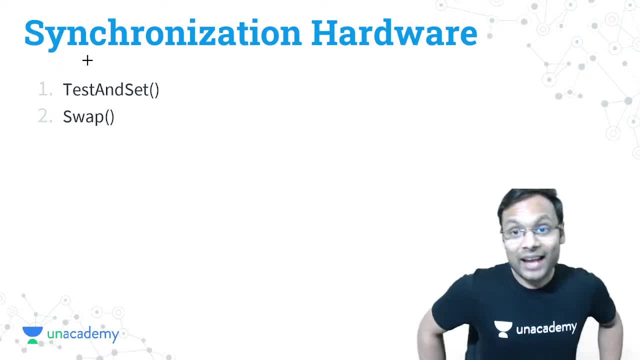 computer architect means the computer designer, the person who designs the cpu, who decides that a cpu can execute or can support what type of instructions. so if that particular person, architect, decides that let's give some kind of instruction support, let's give some kind of instruction support, those instructions can be. those instructions can be used or utilized for synchronization. 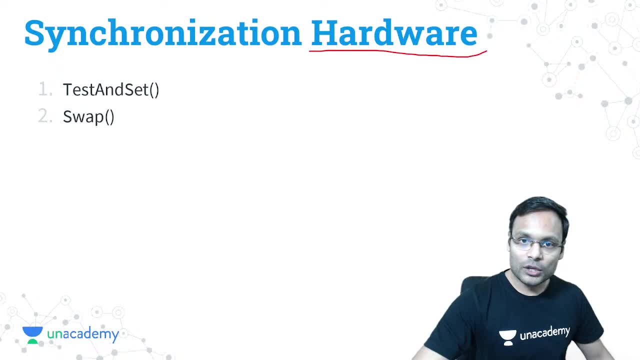 then we talk about synchronization hardware. so hardware is nothing, but we will be having cpu and those cpus will be able to execute the instructions. what type these type? so the architect will design a cpu in which we will be having certain instructions. those instructions your process or program can use to provide the synchronization. that is why 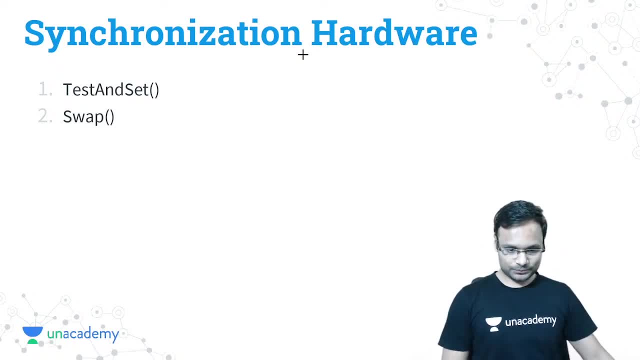 hardware. that is why hardware- okay now synchronization hardware. you understand what is the meaning of hardware. here we will have instruction support by cpu. those instructions can be used for, can be used to provide synchronization. all those members here, there is a new educator joining our team. if you don't know about that, tomorrow 9 pm i am going. 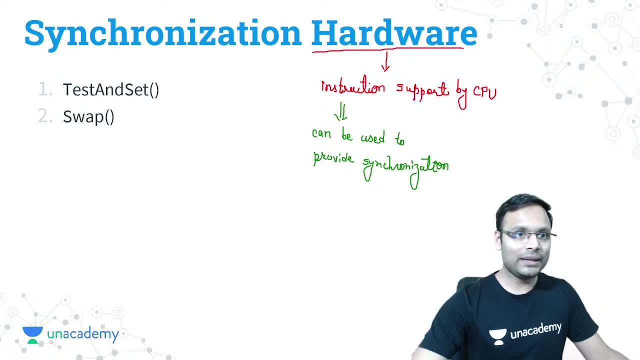 live and launching the cpu. so if you are new to the cpu, please do not forget to subscribe to the channel and i will see you in the next video. bye, bye. a new educator for this particular channel. okay, fine, understood. but if we have such kind of instructions supported by cpu, and these are the utilized, or these are utilized for the 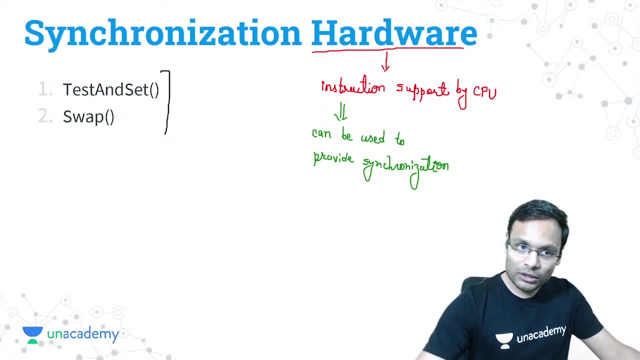 synchronization. these instructions cannot be normal instruction. no user process cannot execute in the user mode these instructions. these instructions should be privileged instruction which should be executed in the kernel mode, right? so i am writing here, srq, just because, just because these are those instructions which are to be providing, or which are going to provide, the synchronization. that's why should be. 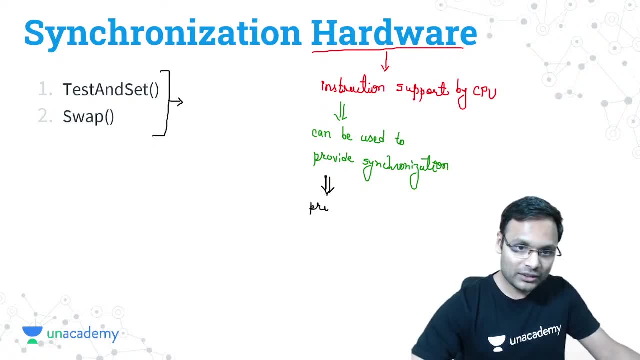 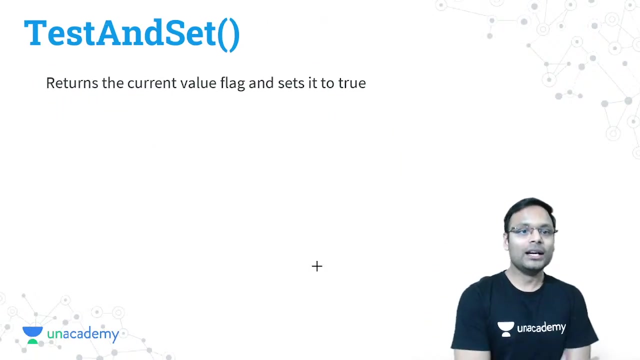 privileged type instruction. so i am writing: these are privileged instruction languages. what so? t is first section. what is testindset, what is test? and it's not okay, check this here. first word, it will test something, that, what is the value, and after that it will set also something. 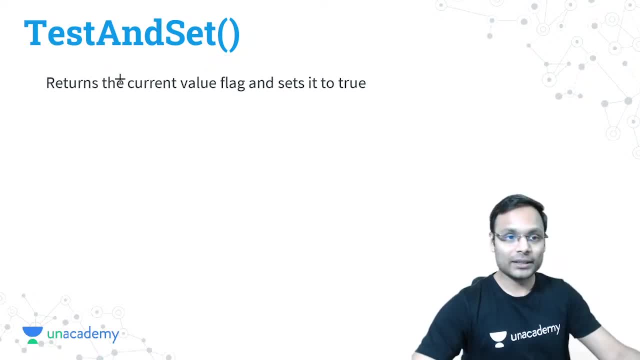 by something. what is that particular test and set? so it test that whatever you are sending as a parameter, that value is what? true or false? if you are having such kind of, you are having such kind of test and set, you will call test and set with some kind of variable boolean type, some boolean. 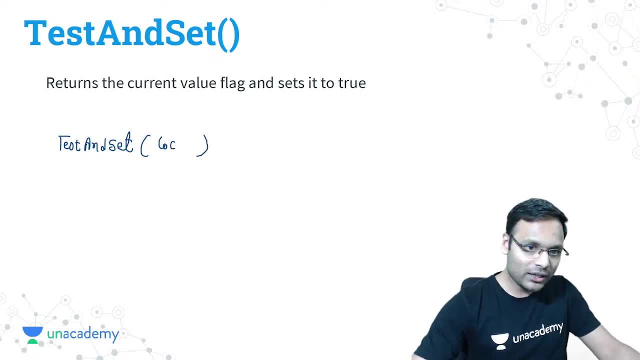 variable you will use. let's say you have called with lock, lock is initially whatever, false, true, whatever you will, you will initialize the locker value based on the implementation. so when you call test and set for this lock or some boolean variable, it returns the same value, whatever. whatever the value you have. if lock is true, it will return true if lock. 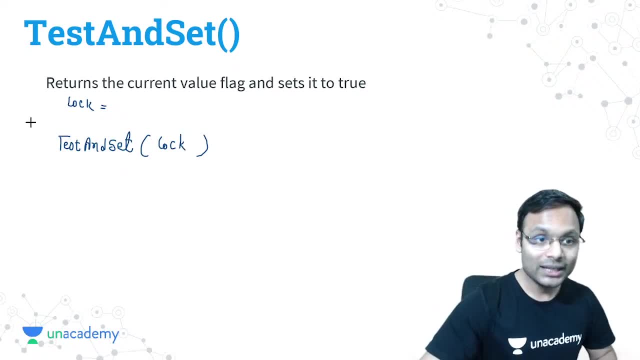 is currently false, it will return false. the function will return what? exactly the same value of parameter which you are passing. if it is true, it will return true, lock, test and set. if it is false, then it will return false, but before returning, before returning this test and set. 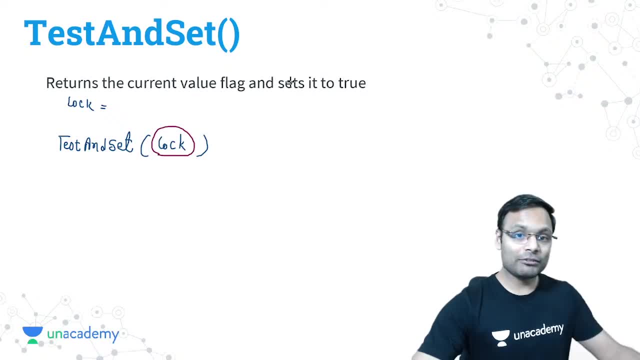 will set also what it will set. it will set the value by true, so lock is initially false or true doesn't matter. it will set lock to true and whatever the previous value you had in the lock, that will be returned by test and set now exactly how it will impact your. 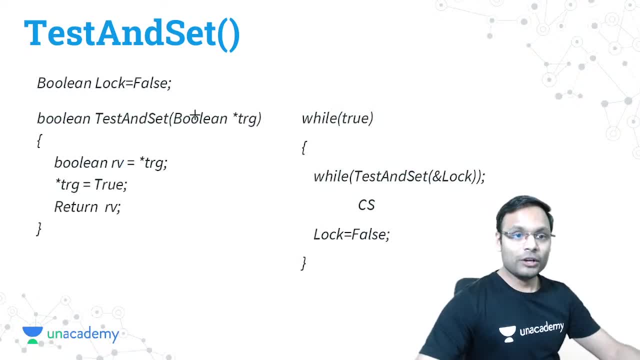 synchronization. so first of all we will try to understand how this test and set works. so look at this. we have a lock variable. let me say: initialize with false. we will see by false. so what it is doing. whenever you are calling the test and set, it will first it. it is being called. 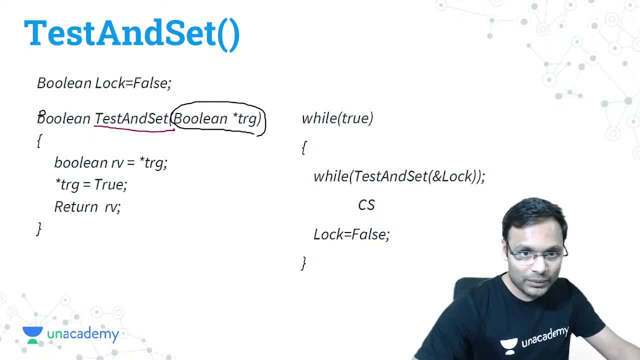 by some parameter. you have called with some parameter, that parameter, you have catch. you have caught in a point, the triangle, what you are copying this parameter as it is in a variable RV. why? just because if the value with which you have called the test and said it is true, it will return. 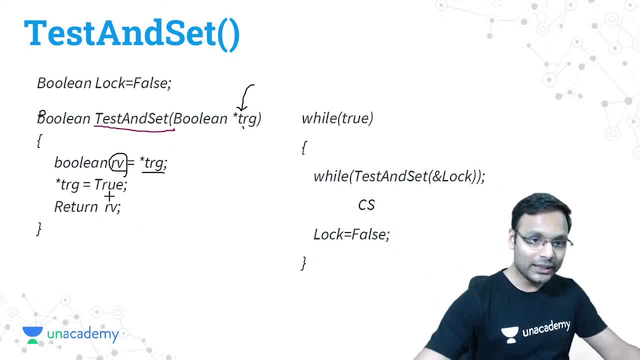 to. if false, then it will return false. so what you did? you have copied that value in some result, some particular variable, RV. okay, after that, what? after that it will set the value by true and then return that over value which you have preserved in RV. so this is the work of this: test and set 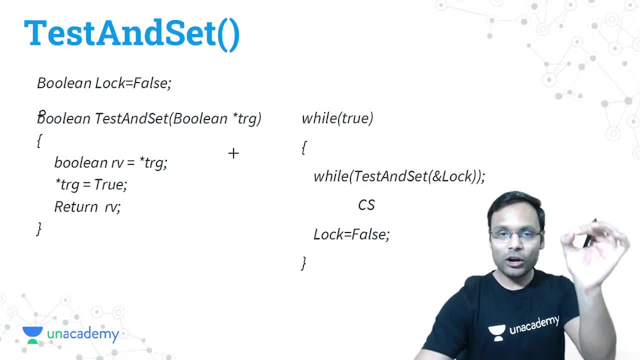 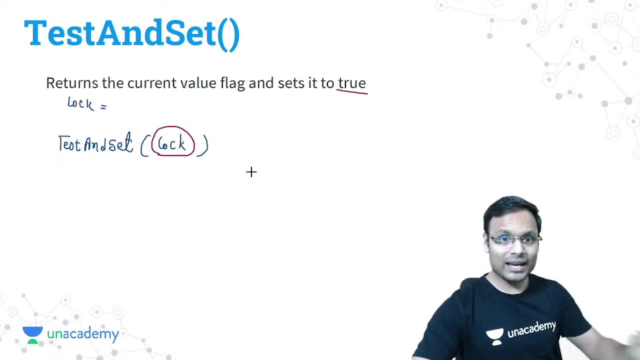 exactly the same thing I told. whatever the parameter you have called with previous value, I have preserved in RV so that I can return it same value, either true or false, but before that I am setting it to true. if you remember, if you remember yesterday's lock variable example in the lock variable example, 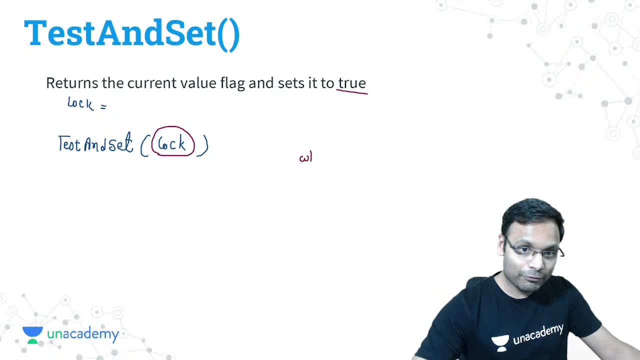 what was happening in the process. we were first checking if lock is true or false. if lock was false, we were going ahead. we were going ahead and we were setting lock by true. that was the lock solution. but this solution could not work. this solution could not work. why, sir? just because we were able to. we. 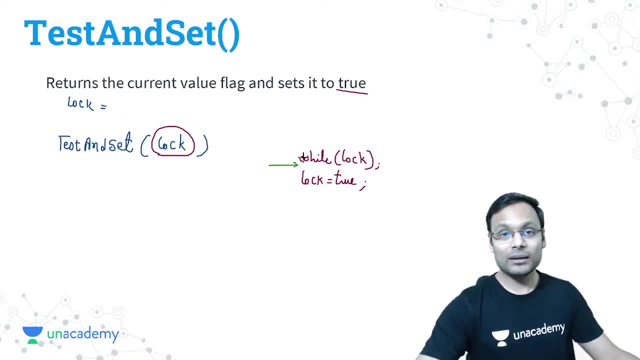 were able to have a preemption in between this. what is the? what is the preemption at that level? we were able to preemption, preempt the process, what we have checked the lock: it was false. yes, we should go inside the critical section, but before that we will have to set that. 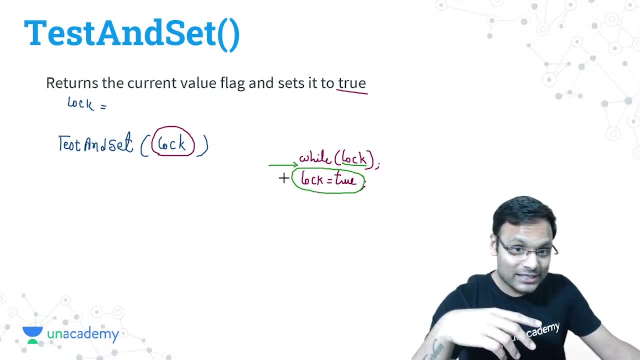 lock is equal to true. yes, but before this setting lock equals to true, we were able to stop the process execution. that is why this lock variable was not working. I'll have to check. if lock is false, I can go inside the critical section. but before I go into the critical section I will have to set lock. 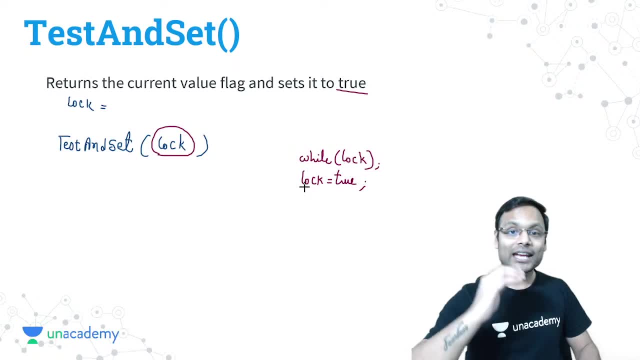 to true these two things. I have to do in such a way that I cannot have any preemption, but I was able to have preemption. that is why the problem occurred yesterday. today we are going to eliminate that preemption kessay, we are going to check lock, yes, and after that we are going to set the. 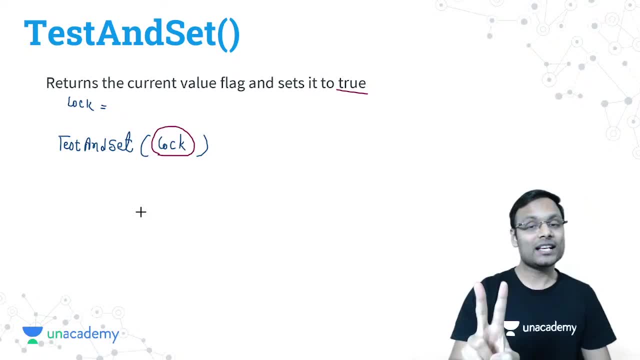 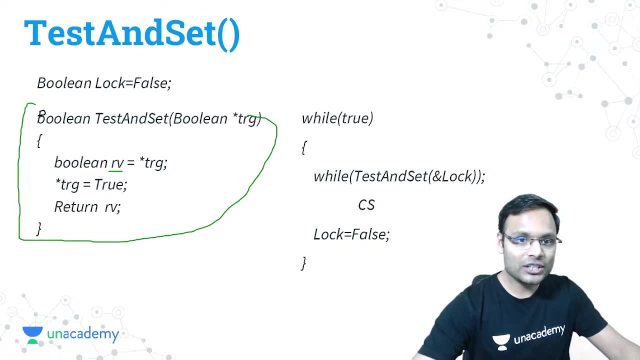 lock by true. also. yes, in the same function. test and set. yes, and this is is not actually a function, it's a synchronization, hardware execution, and that will be, or atomic, that will be atomic. now, what is the atomic meaning, sir? atomic means either it will be completely executing or it will never be executed. there will not be any middle case. you cannot have. 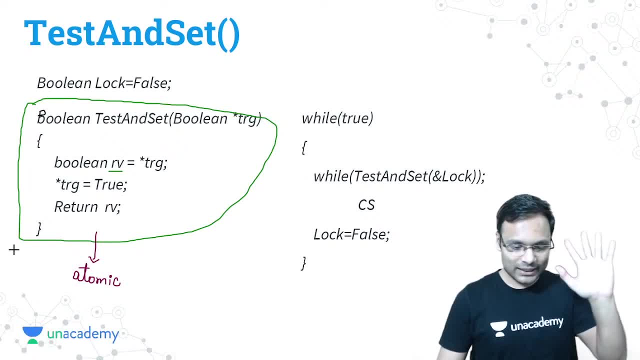 a preemption in between. like that way, you cannot set a parameter in between or you cannot preempt, you cannot have the preemption in between. so what happens? we will check the lock, yes, whatever the lock value is there. if it is true, we will return true. if it is false, we. 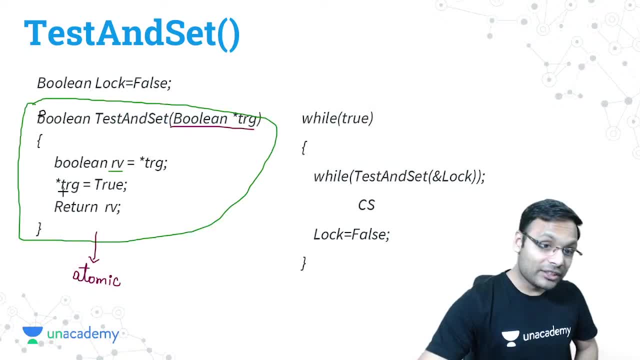 will return false, like yesterday we were doing, but after that we had to set the lock- is equal. yes, both the things we will have to do in such a way that there cannot be any preemption in between, and that is what the idea about giving this execution as atomic in the hardware. so how the process will. 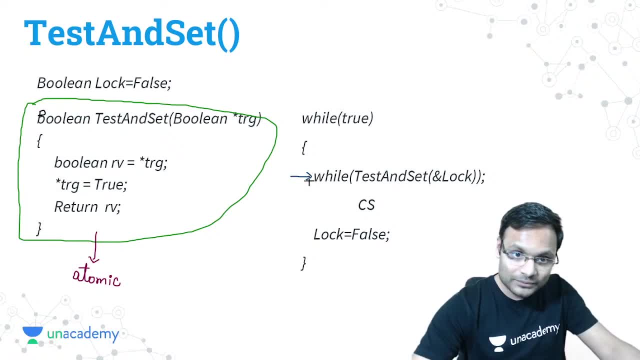 look like process will look like process will execute this while in the while we will test that the lock is true or false. so what we are doing is we are calling test and set with lock address. why we are calling test and set will lock our address so that we can make the changes in the. 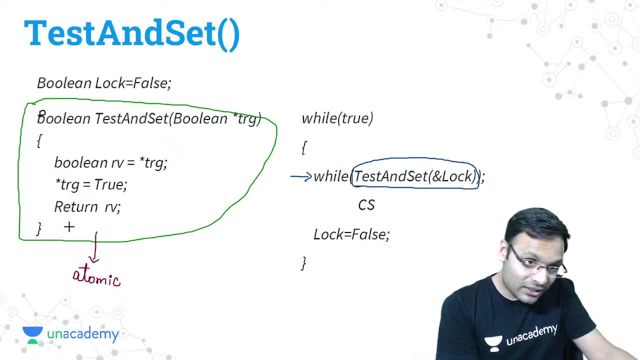 lock. if lock is false, this return false. if lock is true, this returns true. so, initially, lock is false, it returns false. yes, and along with that it makes this lock is equal to true. so both the things are done in atomic way. you cannot have a preemption. yes, this solution works perfectly. 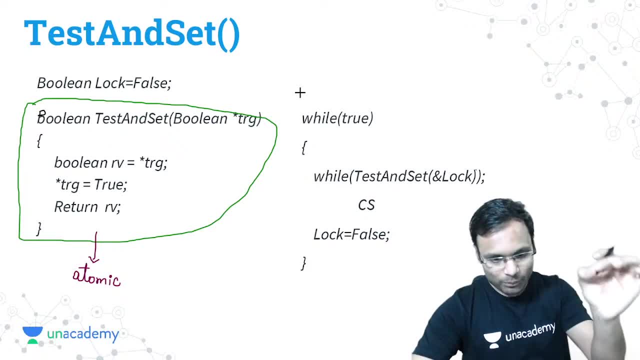 fine, this may. mutual exclusion: cop problem nahi ayega. every process which will try to use this test and set for the preemption- sorry for the synchronization- will have such kind of code, p0 also and p1 also, same to same code. so let's say, if p1, p0 wants to go into critical section. 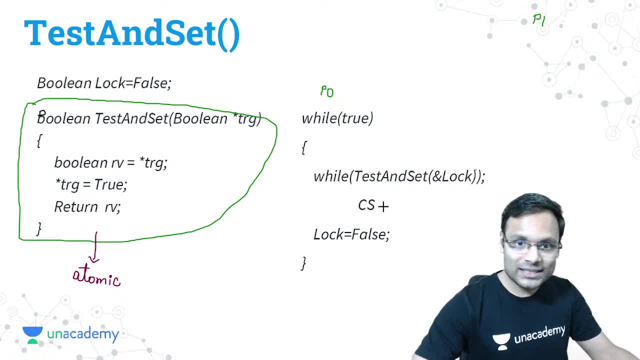 initially, lock is equal to false. yes, check, test and set lock. we have sent lock value here. okay, is pointing to lock, which is false. so what? we will copy value false in the rv and this is equal to true. so we will make the changes in the original variable equal to true and after that we will. 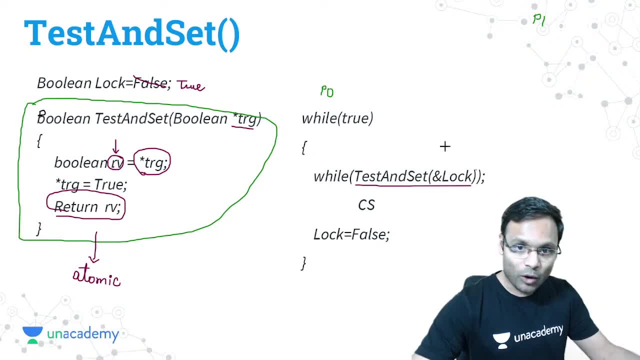 return the preserved value false in rv. so what this returns false. this will be completely executed. after that you can have the preemption, but you will have to check the condition while immediately. you will check the condition while it says false. this value is true. yes, you can go inside. 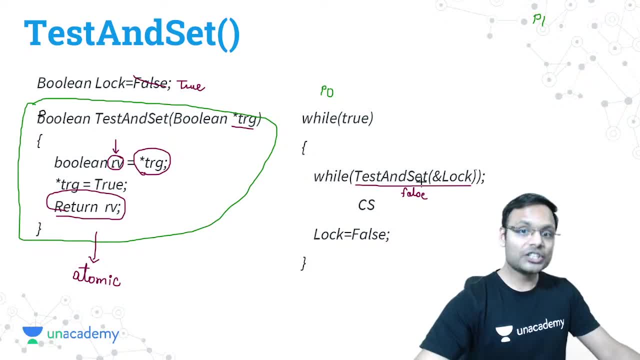 you can go inside. so while condition gets false means you are not going to stuck here. no semicolon means if condition is true, you will be stuck here only and continuously, and you can go inside when the condition is false and lock is true now, if any other process. 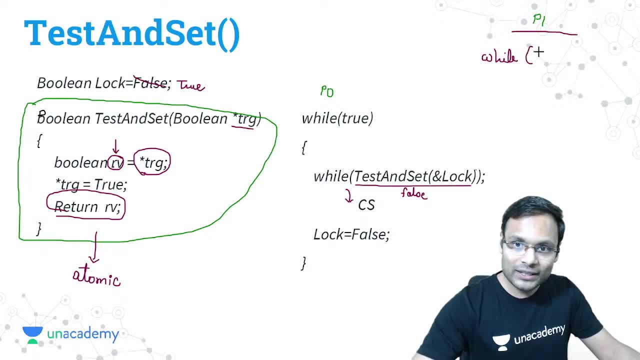 p1 what you will do. if it wants to execute and it wants to go into critical section. what it will do? it will run the same test and set lock. now what happens? this particular lock is true yes. so when we will send, lock is equal to true. this rv will receive true yes. it sets to true yes, and after that it. 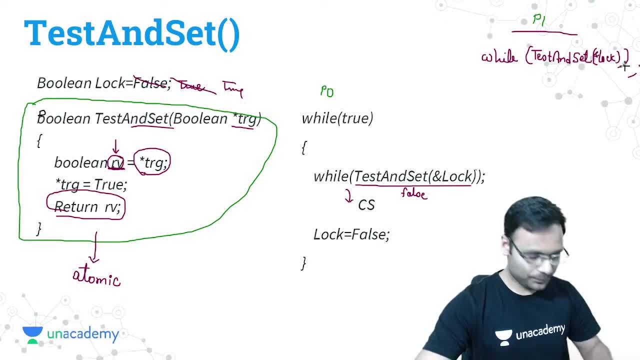 returns true value: yes, p1 will stuck here. only in this true, only it will stuck. p1 will stuck here. yes, p1 cannot go further. no, why, why? why can't during that? so that? why? just because lock isn't Now through, so P1 cannot go ahead. 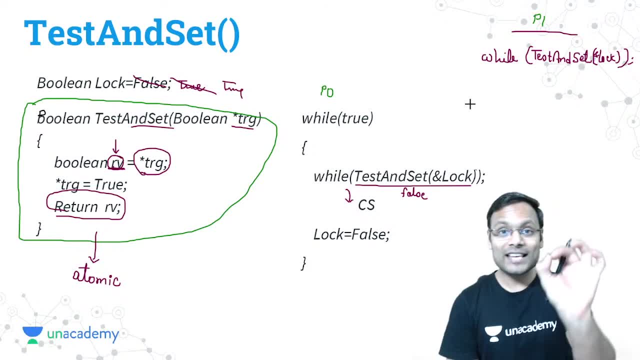 But p1 is executing. yes, p1, he is executing that while loop and he and and he. if he is executing but it cannot go ahead, means P1 waiting for the Critical section. yes, when P1 is executing, Meaning p0 releases the critical section, makes the lock is equal to false in the exit section after that. 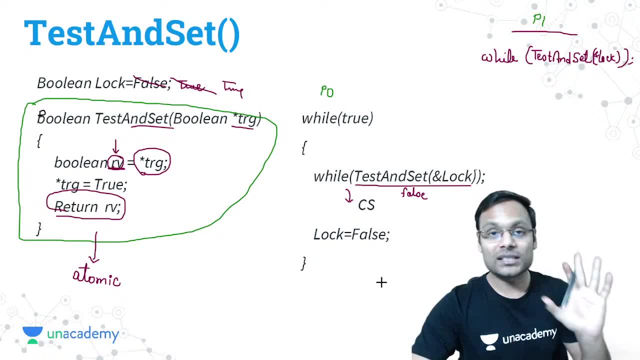 only p1 can go ahead. yes, so p1 is waiting. yes, but executing also. p1 is executing in cpu and executing this statement while again, and again, and again. but p1 is not able to have a particular, you know critical section access. why? just because we have made our p1 to stay here until p0 comes. 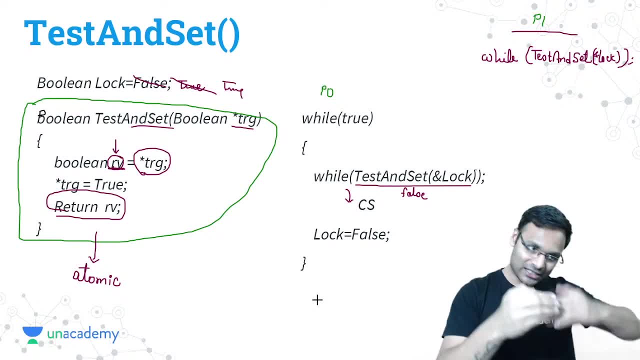 out and this particular case when p1 is executing on cpu but p1 cannot enter into critical section or cannot have a progress further. progress means cannot execute further. this particular situation is called as busy waiting. p1 is executing means busy, but still it is waiting for critical. 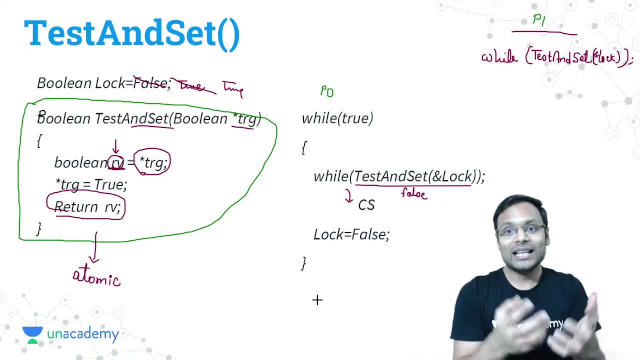 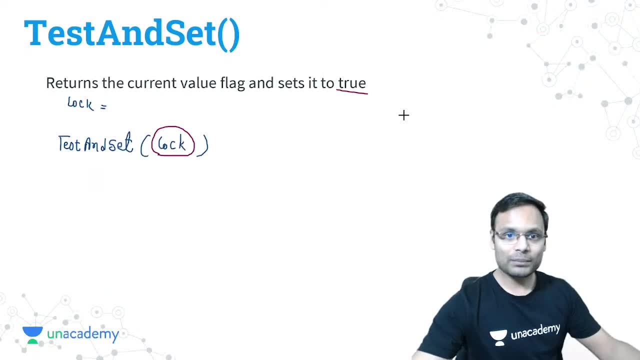 section access. why? just because we have made our p1 to stay here until p0 comes out and this particular section and executing that, while the condition again and again and again that is busy waiting. understood this? so i am writing that particular definition here: busy waiting is what? 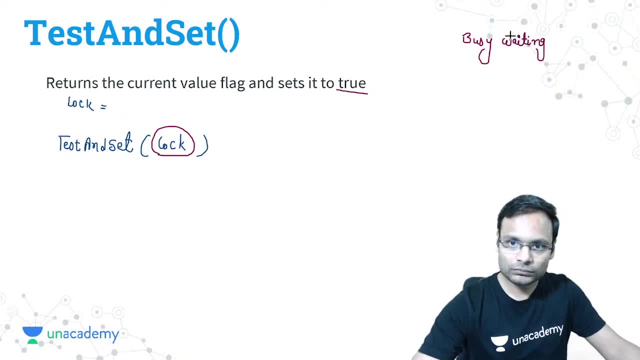 a process executes. a process executes on cpu but cannot go further because of critical section. solution means it is stuck over there. then is not the last key where you can have the correct expression under which you have to write the process process. this button is substance. is this one? 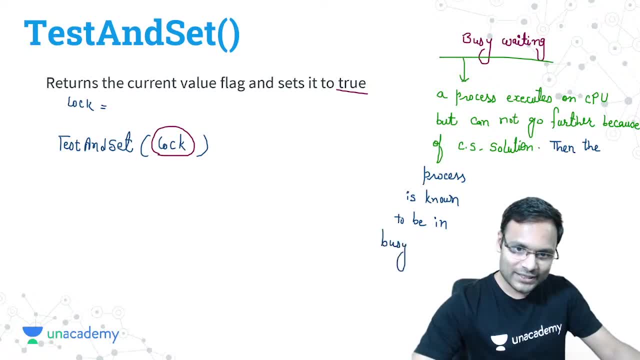 the process is known to be in busy the process. now notice this question will come as it is in exams. what, within 6 hours, they will additional question they give to you? then they will help you a lot anyway. what are they going to do? so how many questions would they ask you in exams? 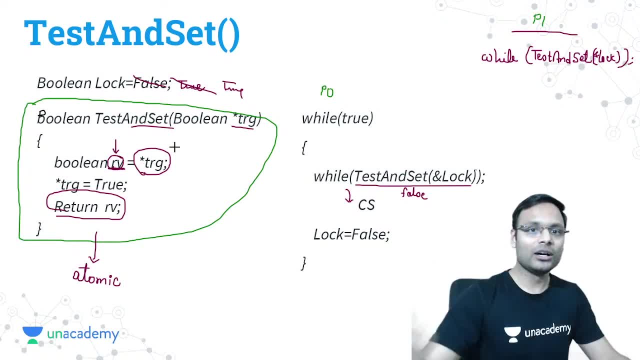 really they are giving back to you that little opportunity will be enough for that. in your exams. have certain changes in the code and then they will ask how this particular code can work. you can easily answer yes, why? just because if you understand the code and how it is running. 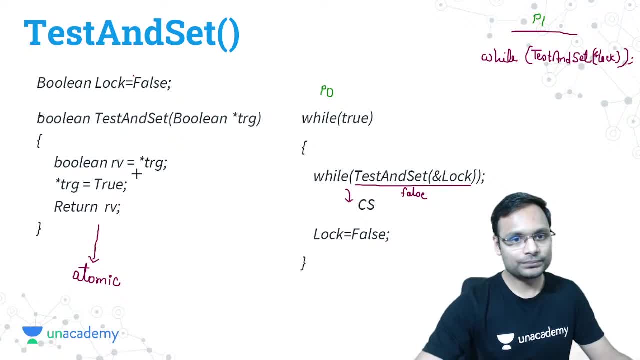 you can easily answer around questions. suppose: what if lock is initialized with true? what happens? what kind of changes you can make in this test and set or in this p0 process execution so that you can- you can make this particular solution work. how you will do that. you will. 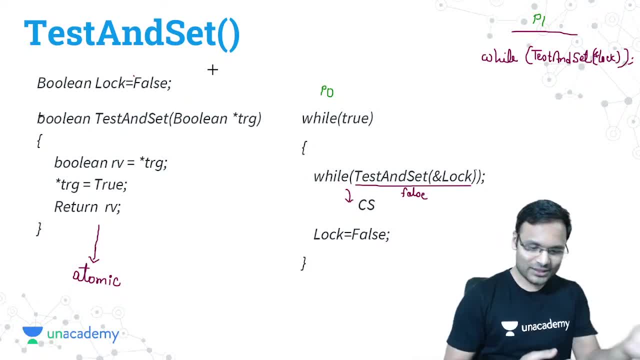 have to understand it. so such kind of question may be asked and you can solve. of course you can solve if you understand how this particular solution is working. it's exactly same as lock variable solution instead of lock variable checking, while in the, in the while lock variable checking and. 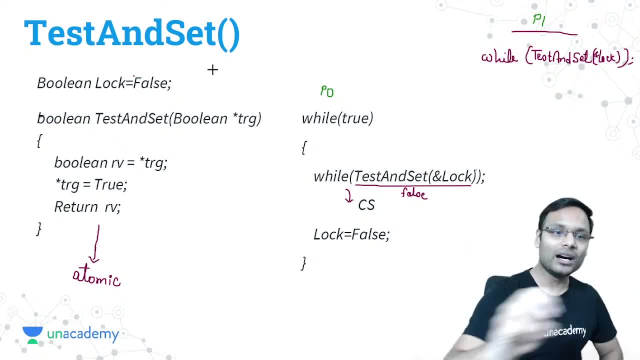 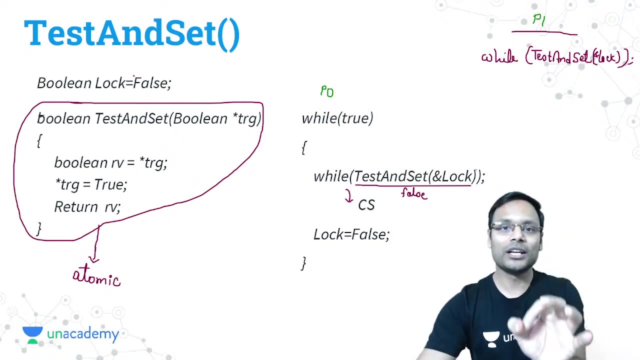 lock is equal to true these two statements. we have merged in a particular instruction which is hardware running, which the hardware running and it can made or it can be made as atomic, so that we cannot have preemption in between means. we will ensure the mutual exclusion, error combination, celebratory project. and this is the important question: what is? 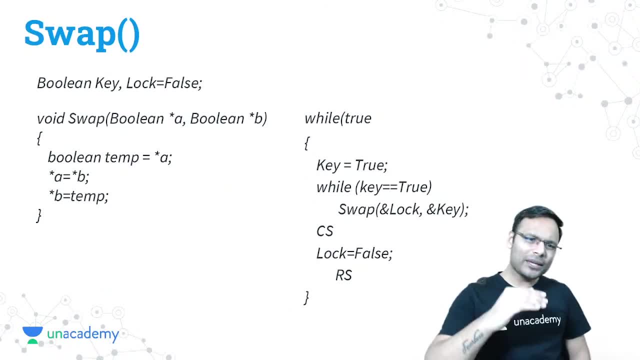 a, so you must solve. you are not doing your job, inania, since you have been working in the code from beginning of this step till now- variable in such a way that initially the lock will be false. when lock is false, process can enter into critical section. if lock is equal to 2, the process cannot enter into critical section. 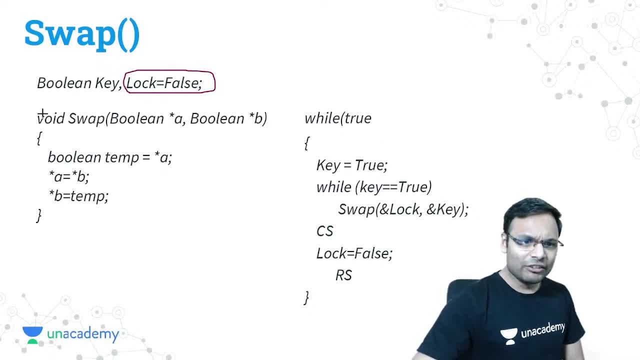 very simple: same to same as lock variable, but here we have made a swap function and that atomic function that to atomic function, right. so if you want to provide any kind of solution to synchronization, of course your process will use the synchronization solution. right now synchronization can be totally software, like yesterday we have seen only software instructions you are executing. 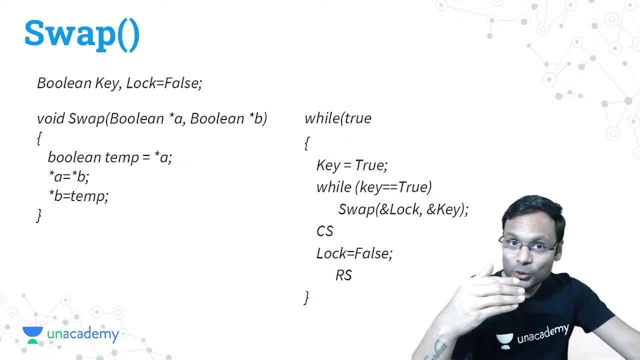 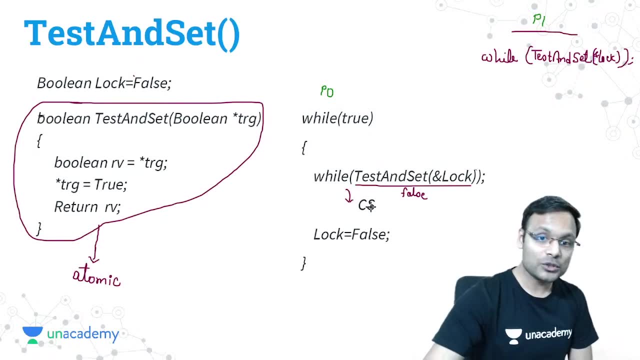 or software statement you are executing, or the synchronization can be provided by using such kind of instructions. so this type of solution is hardware. why? just because actual synchronization is provided by testinset. that is why we call it as hardware solution and testinset is a instruction. right here we have a swap function that swap. 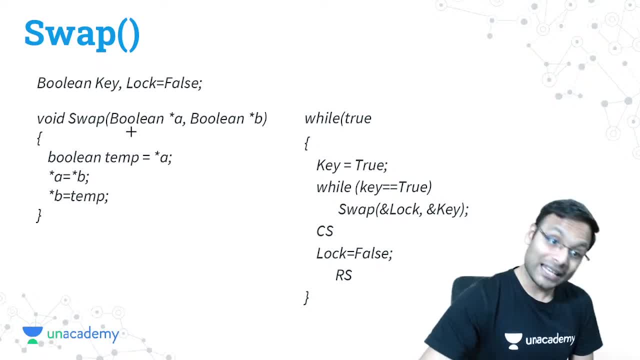 function does what swap function swaps two values in actual. yes, that is why we are using the pointers. so two boolean variables address we will send here. those addresses will be caught in the pointers and you know that how to write the swapping right, which one means programming, say so: boolean temp is equal to star a star is equal to star b star. 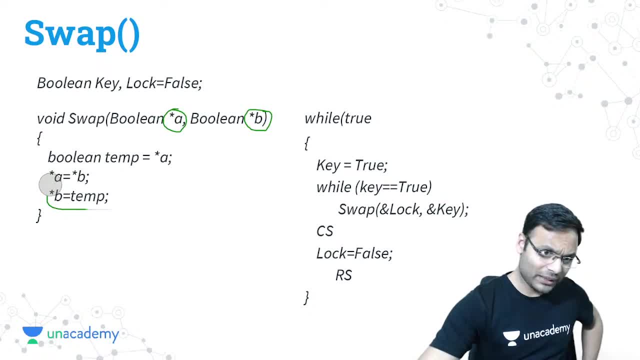 b is equal to temp. this is the swapping. what exactly this swapping does? this swapping is actually making my processes go ahead in the critical section. if lock is initially false, now let's see here: initially you are executing this function for a process, let's say p zero. 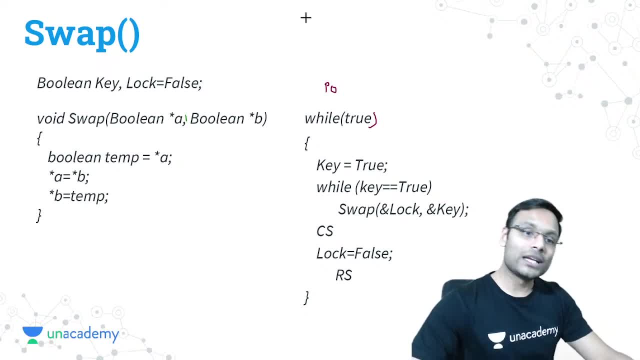 now p zero is running this. let's say p zero goes inside the critical section. how let me write all those variables? two variables here: key and lock. we have made keys equal to true. that is initially true. okay, after that let's check out this condition. while key is equal to equal to true, key is equal. 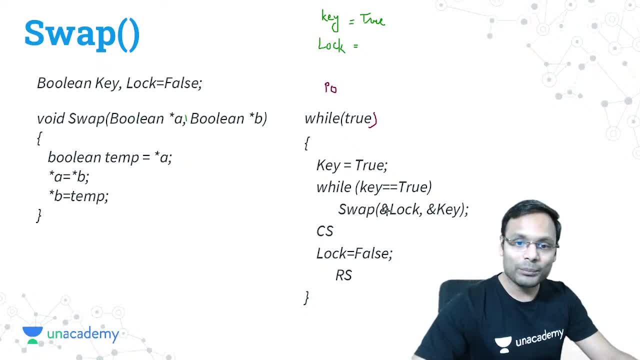 to equal to true. yes, then make swap between lock and key. so lock was initially false, key i have initialized with true, yes. then call swap. when you swap, what happens? this becomes false. this becomes true. done after that you check again: key is equal to equal to true. yes, key is equal to equal to true. now what? 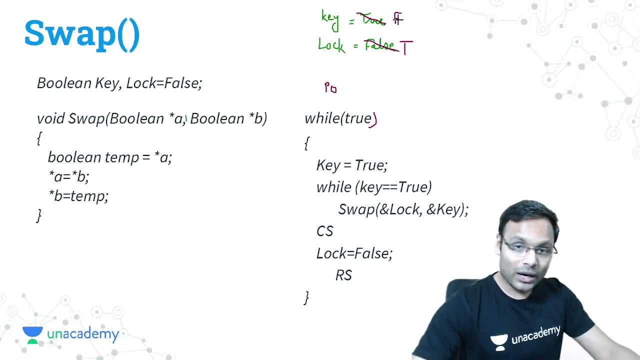 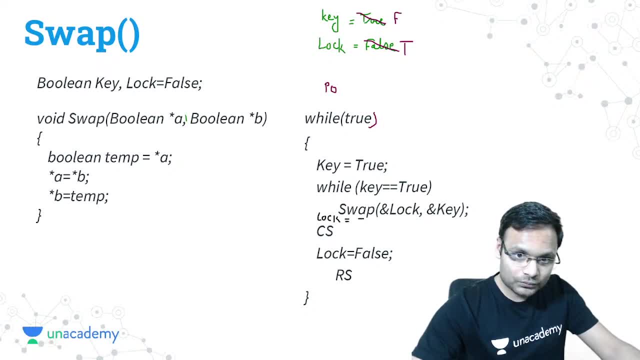 be. lock is equal to true. we will have to keep lock is equal to true here. as soon as we come out of loop. we should make lock is equal to true. why? just because, oops, I am making it wrong. key is equal to true. I will have to make key is equal to true. fine, so I will make. 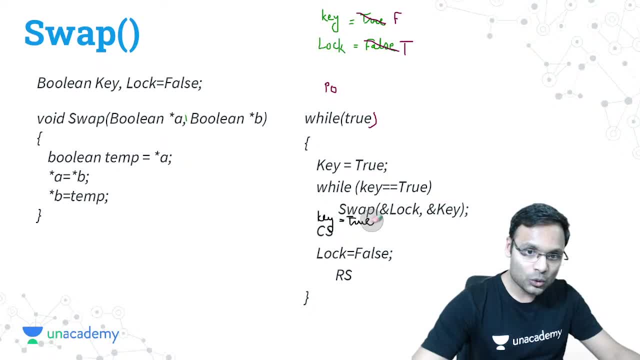 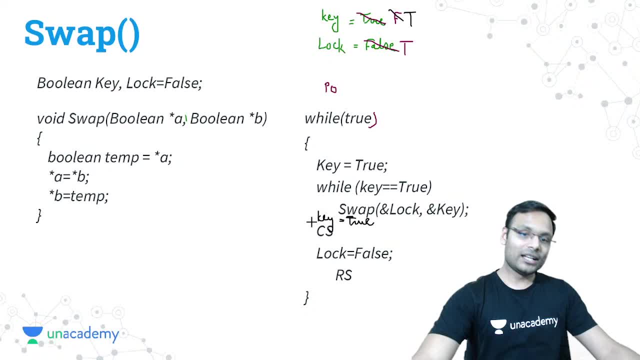 So I made: key is equal to true. both are true. true, yes, now I can enter into critical section. Now I can enter into critical section. if suppose now P1 wants to enter into critical section, what P1 will do? key is equal to true set. then, while key is equal to true, swap, swapping will. 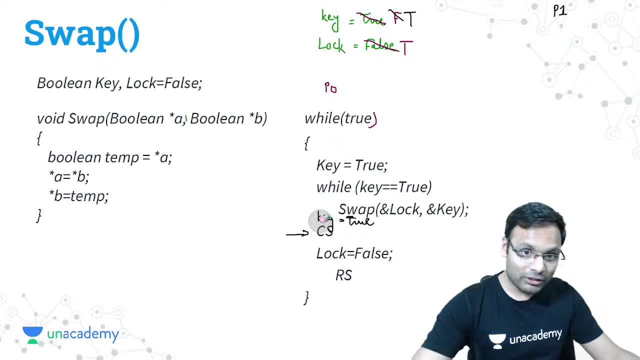 make both true, true, true, true, true. If I will not even make key is equal to true, that will also be fine, no worries at all, why just because any new process comes into the critical section before it wants, or it will go into critical section, it will have this key is equal to true. 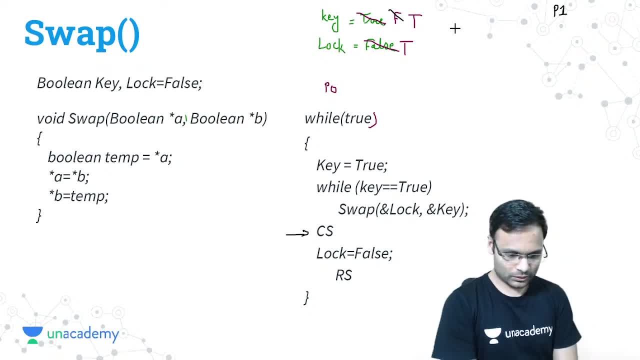 anyway, anyway, right. So this P1 comes, makes key is equal to true, yes, while key is equal to equal to true. So true, yes, swap. this will be swapped, becomes true and true only, and this P1 will stuck here only in the swap. P1 will stuck here only in the swap. why? just because? just because both. 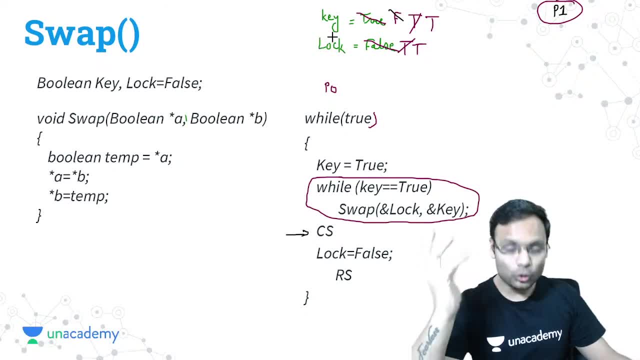 key also and lock also: true, true, Dono, true, true hai. toh koi tension nahi. Ok, let me commit, come again. once again I will explain. fine, let us say P0 wants to execute, So P1 will start. fine, what is the key? nothing, lock, false. Ok, great, P0 executes, it says: key is: 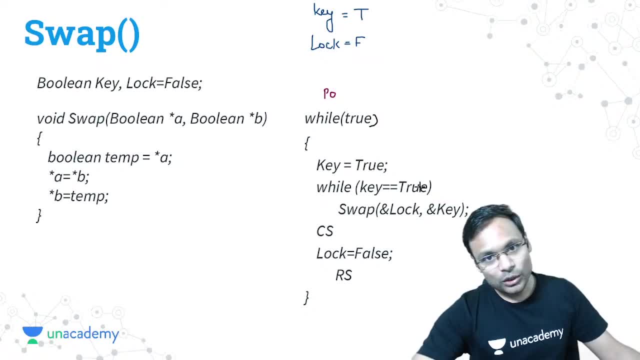 equal to true. fine, while key is equal to equal to true, yes, loop and loop says swap. in the loop, execution is swap, So we will swap these values. it becomes true and key becomes false. we will go inside. key is equal to equal to true. 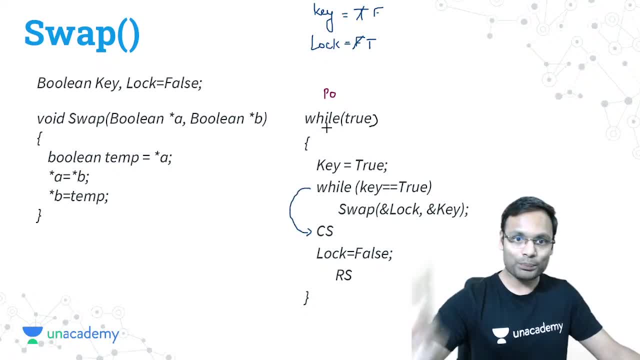 No, false. go inside critical section. So P0 is in critical section. Now next is: what next is this? P1 comes into the critical section. P1 executes the same yes key is equal to true. it makes key is equal to true. After that, while key is equal to equal to true, yes, swap. 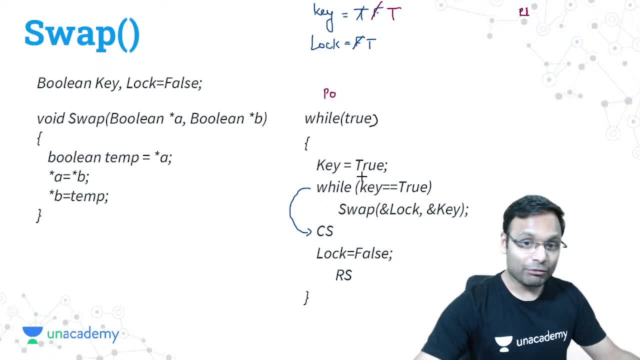 both are true. yes, keep swapping, keep swapping. if we will keep swapping, true and true will be swapped, swapped, swapped. P1 cannot enter into critical section until we make the lock is equal to false again right, But here we have a problem. what is the problem if we can? 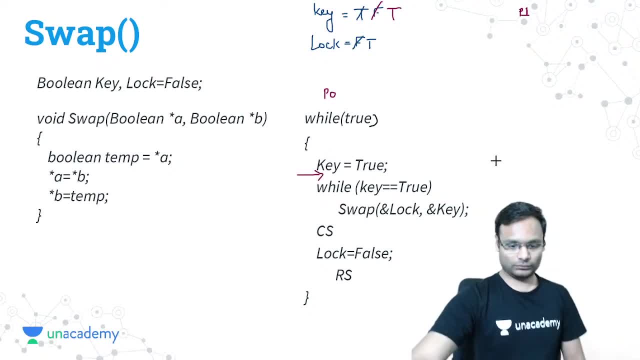 preempt this function here. if we can preempt this function here, then we can have a problem. problem is, what problem is what I will tell you. I will tell you. I will tell you. Let me go to the original state. initially key nothing. yes, calls for lock is equal to. 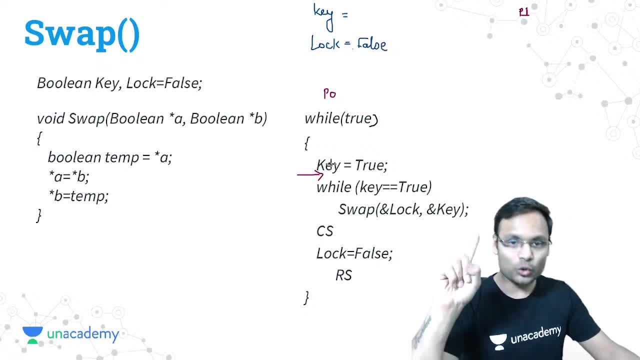 false. ok. P0 executes only first statement. key is equal to true, done and P0 preempted. here I am making preemption. what happens next? P1 runs. P1 runs for P1. key is true. lock is right now false. P1 also runs this execution. 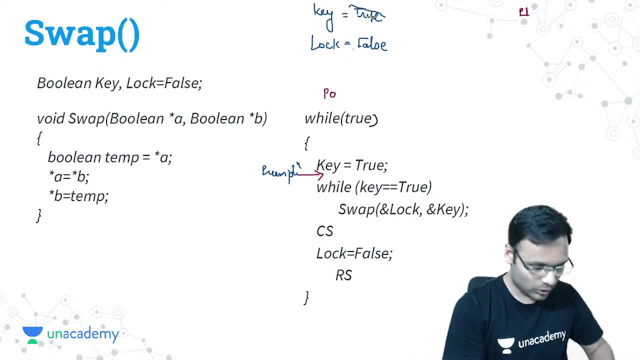 Key is equal to true, so P1 makes key is equal to true. after that, after that, whichever process you want you can go ahead with. let us say you are going with P0 first. P0 executes. next is: while key is equal to it, equal to true. yes, then swap key and key and lock. so this: 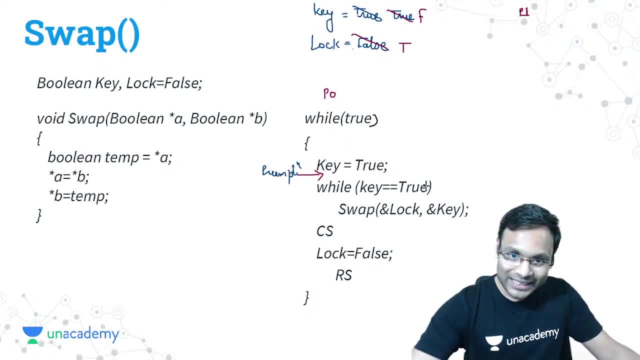 becomes true, this becomes false. While key is equal to equal to true, No condition false. we will come out of the loop and P0 is in critical section. now P1 executes this. while key is equal to equal to true, no, Then the P0 will go. P1 also will go into critical section. P1 will also go into critical section. 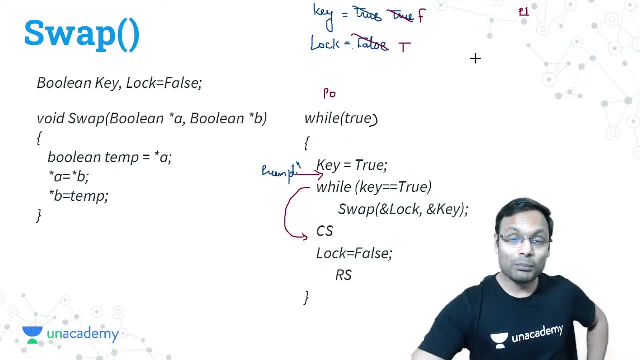 why? just because it is a false value. So it might possible that both processes can go into critical section. understand, yes or no, Yes or no, yes or no. so what we can have here, what we can have here, that is. I hope you understood how P1 and P0 both could enter into critical section, just because because of this key here. 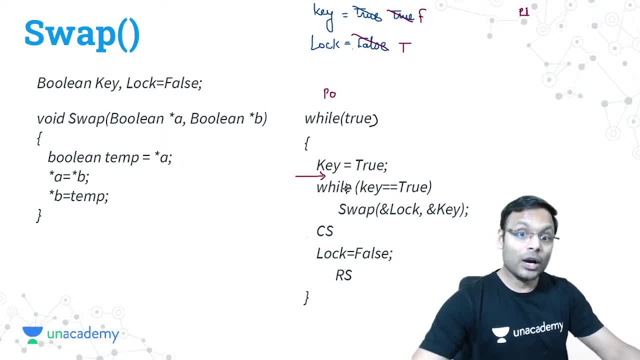 I have made preemption first time of P0. that is why what you can add here is here you can make key is equal to true once again before entering into critical section: enter in before you are entering into critical section: Yes or no In critical section. before that you add a statement here: key is equal to true and check still. 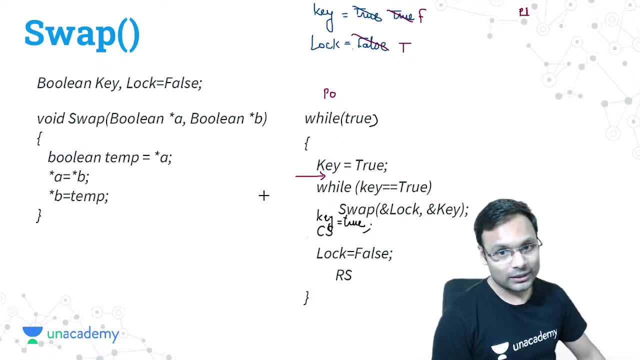 if you are able to make two processes, go ahead or not. check out if you can make and I guess again there will be a problem. and problem is if P0 will have a particular preemption here and again after this while loop before setting key is equal to true again here. 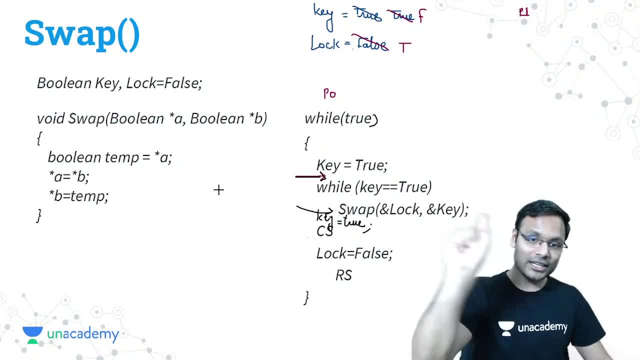 So if P0 will have two preemptions, after key is equal to true and after while loop condition makes false, if you will have preemption, this solution also will make a problem. and problem is what? no mutual exclusion. No mutual exclusion if Preemption happens in process. though this swap execution is atomic between swap. I am 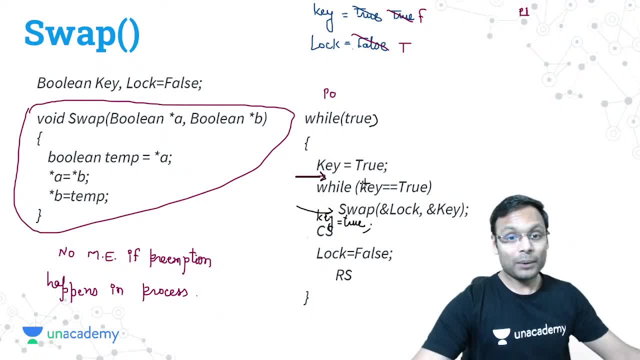 not. I am not able to stop right, but between these statements I can have the preemption yes, possible. So if those preemptions are there still, you will have the what? No, No, No, No, No, No, Not possible. 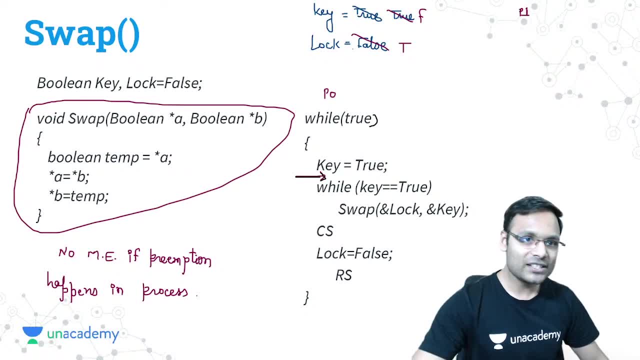 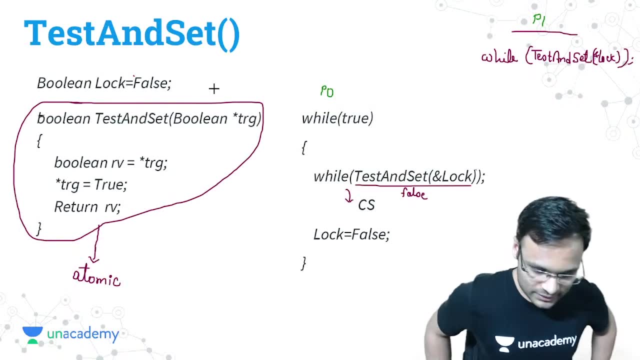 This, rather, there is no parking because of test insert is non-identifiable, ABCD is not possible. This rather, you will have P0. So there will be one. you will have P0 will give you P0. If P0 is proceeds in this way, that this should be it by some, so that there is no actually. 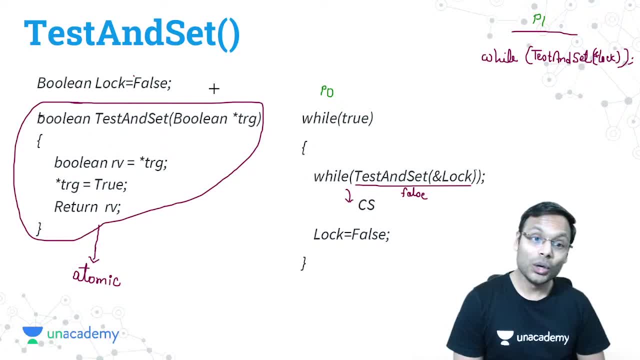 any fitness of it. If P0 has no influence, Feely, Feely, you have P0. be able to solve it? if not, then we will solve it later. later means whenever the actual time comes, when you will be able to understand the synchronization. what is the deadlock? how to? 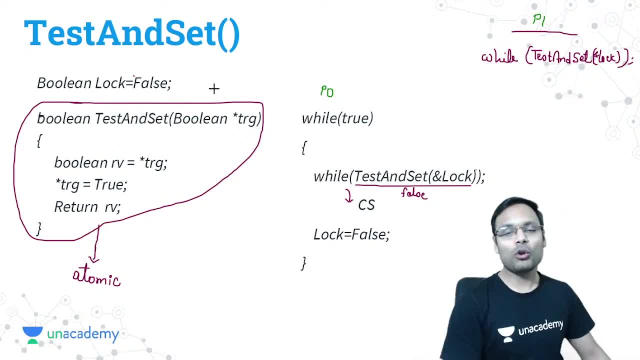 detect that there is a deadlock or not. after that we will solve all these questions so that you can have a better clarity of the topic that how to solve the question. right now you don't know how to detect the deadlock or what is the deadlock, then you will not be able to understand how to. 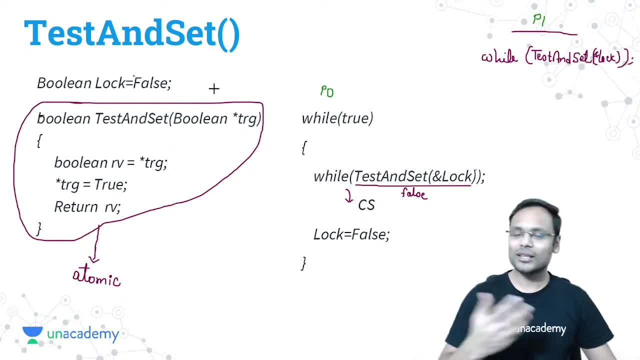 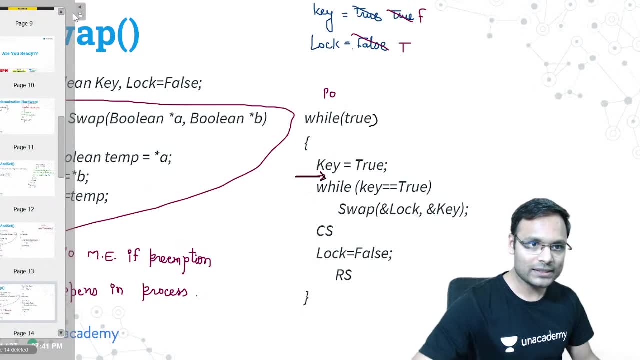 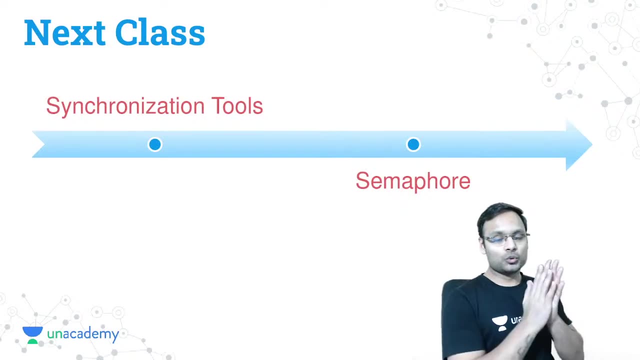 solve such questions if you know that you can solve otherwise, you will leave it fine. okay, there is a mistake here. i'll have to remove this page. blank page, okay, fine. so there are two types of synchronization hardware. we have seen test and set and swap. tomorrow we are going to start a. 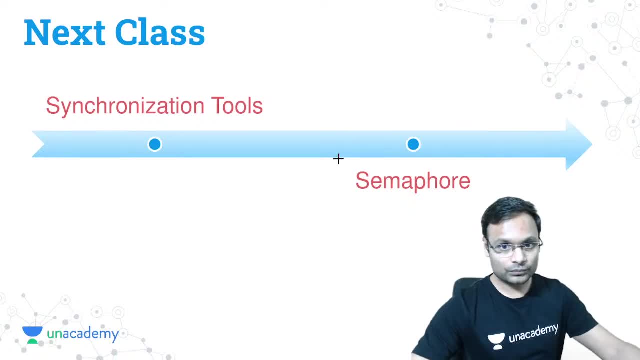 very, very important topic that is sema 4. very important: synchronization 2. so join me in that particular video and i'll see you in the next video. bye, bye, class. it will be very, very important, just because sema 4, if you will understand, there will be so. 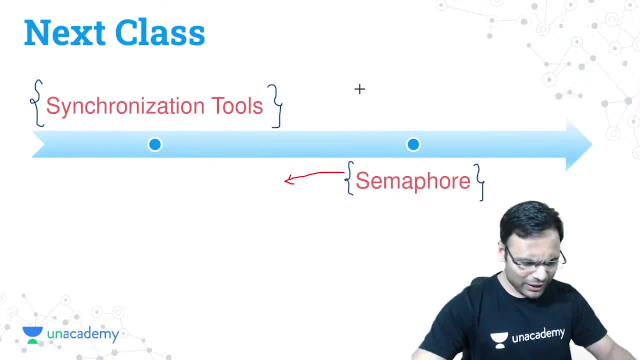 many questions and there are so many questions from this topic. very easy, very easy, very, very easy, very simple and very easy topic. okay, so tomorrow we will start sema 4 and few more classes i am having upcoming, upcoming classes are there. let me just tell you all those classes. 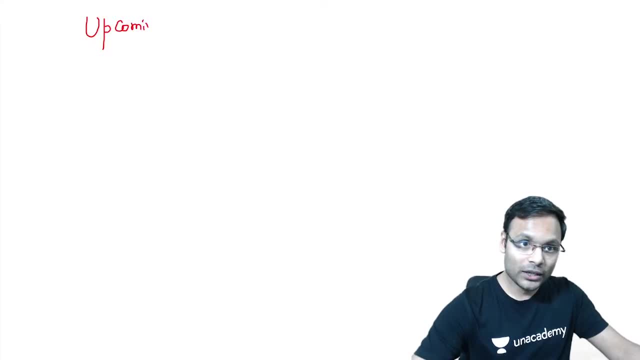 list. so what are the upcoming classes for you? if you guys are preparing for gate, of course you need a better strategy and planning, right? so i am providing you on friday 4 30 pm. i am talking about only youtube. okay, 4 30 pm i am going to give you. 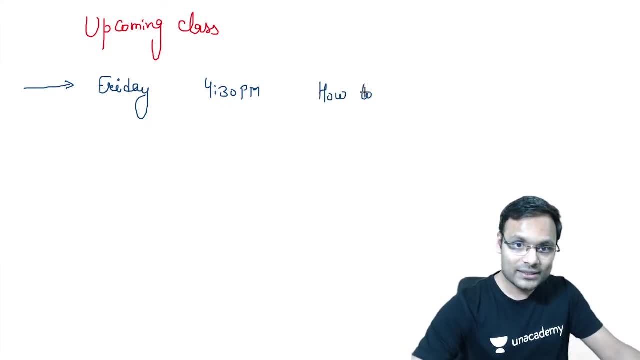 a session, how to utilize remaining seven months for gate preparation. so preparing for gate preparation is going to be very, very important. preparation, a plan strategy, how to utilize the revision, how to go for test series, when to finish the syllabus, and multiple other things. i'll be talking about this then. next one on saturday: 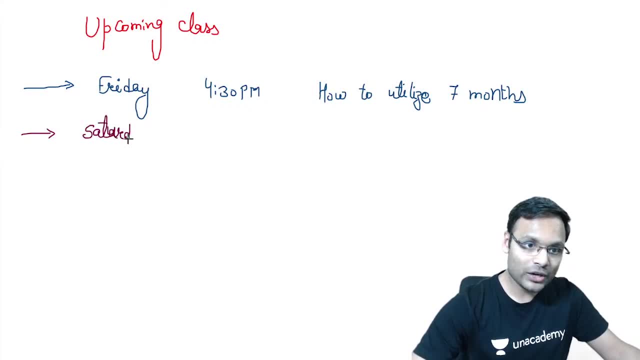 of course you guys are having so many doubts, right? so saturday i'll be having at 12 pm noon a session for you. ask me anything. you guys are having problems, so i am going to give you a session on saturday. i am going to give you a session on saturday. 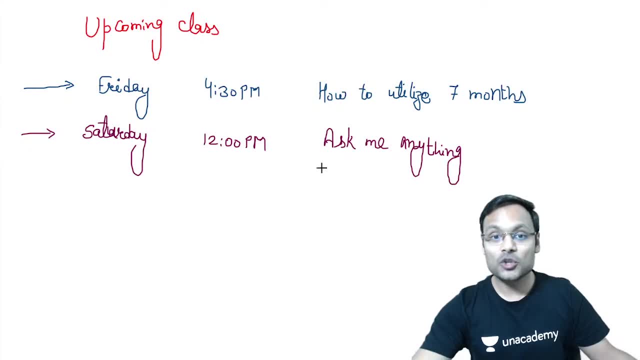 of course you guys are having so many questions and you guys are having. you are having a session youtube. you can come and ask the questions then on saturday only we are having another session. you remember saturday, saturday, nine am. what is there? nine am, we are having a very, very 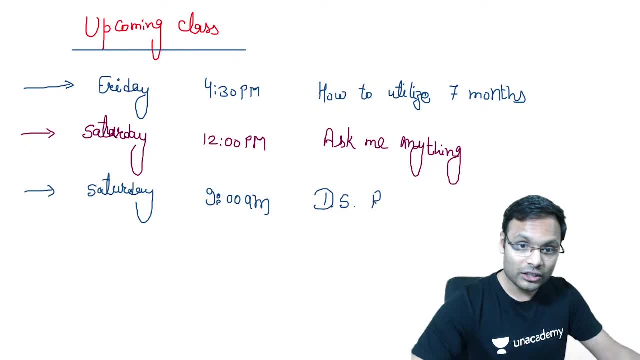 special session. what data structure revision marathon. so these are the sessions upcoming, very, very important. and another thing is, once again i am telling you: tomorrow we are having thursday 9 pm, new educator launch, so his classes will start very, very soon, as soon as, as soon as you will be, as soon. 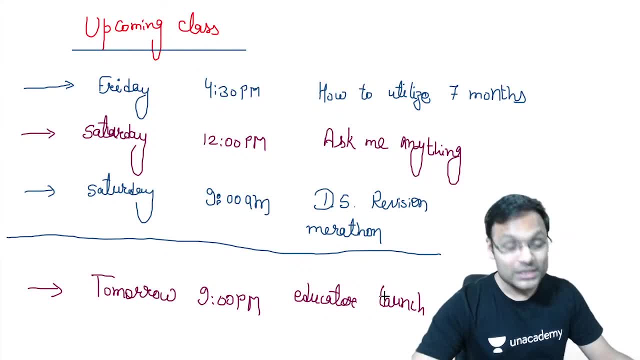 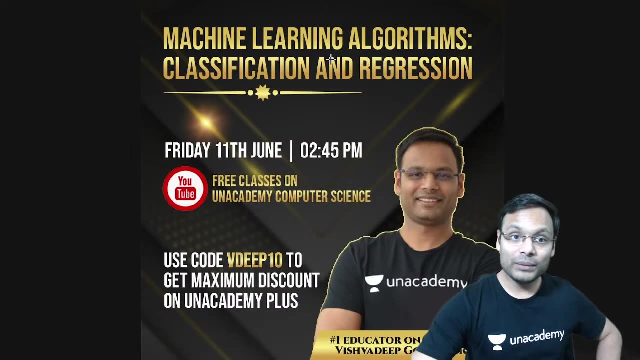 as you will be hearing about who is the educator. you will get the schedule also. that educator will start what course and when and what will be the timing. whoever is learning machine learning, along with it me. I am starting machine learning, classification and regression- very, very important topic, if you. 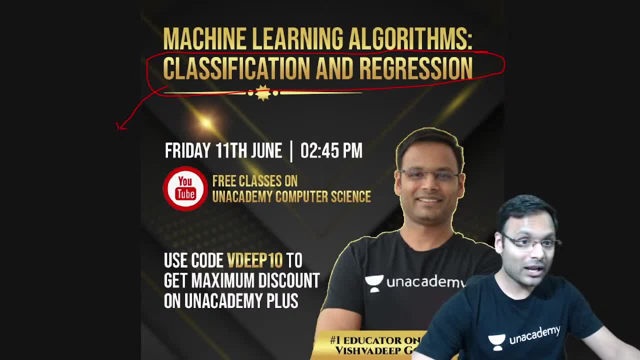 have machine learning in your college also you can learn this. so I'll be starting with theory first, and after that I'll be going for the practical implementation of that. but before that I'll be starting the theoretical part. so at what time? 2: 45 pm, Friday onwards- I am starting this machine. 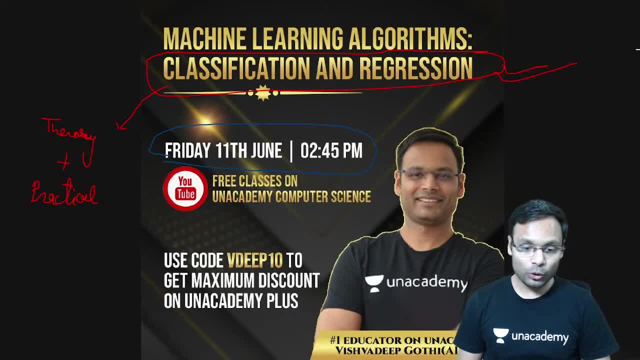 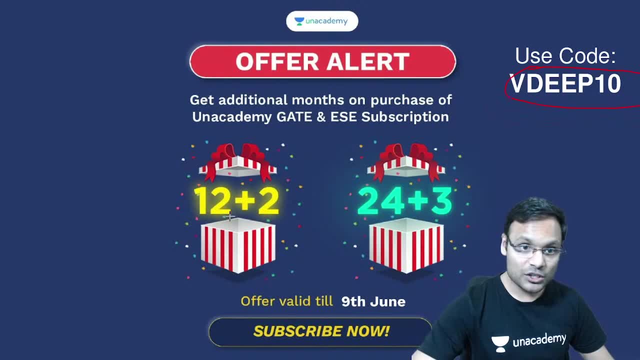 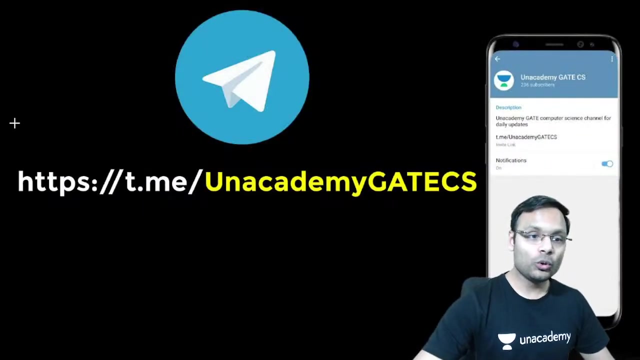 learning, regression and classification. you can follow that particular playlist. anybody who wants to join an academy plus, use this code and join today. why? just because this offer is lasting today, only 12 months subscription. if you take two months extra, 24 months subscription, you take three months extra. you will be getting, if you want to know or get the pdf downloaded. 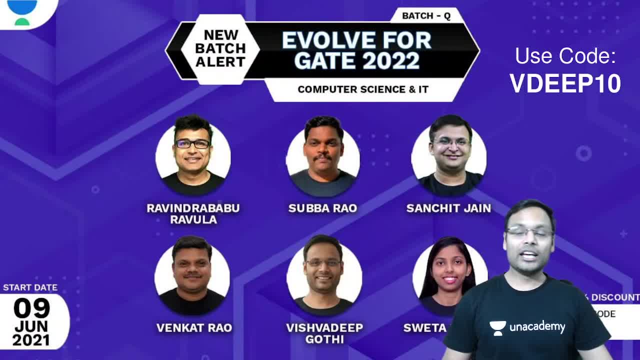 take it from here and you, if you want to join, there is a new batch started today. only look at this. top educators of country are going to cover your syllabus and are going to teach you in the best possible manner. join this just because ascend and evolve batch. this is the last lot of having the full length preparation. 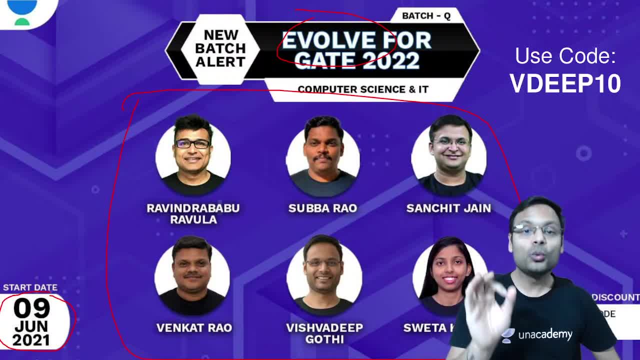 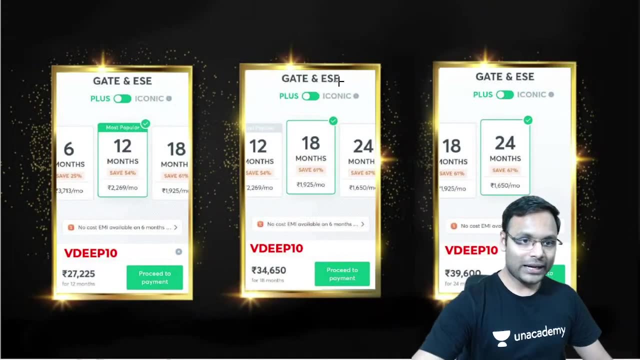 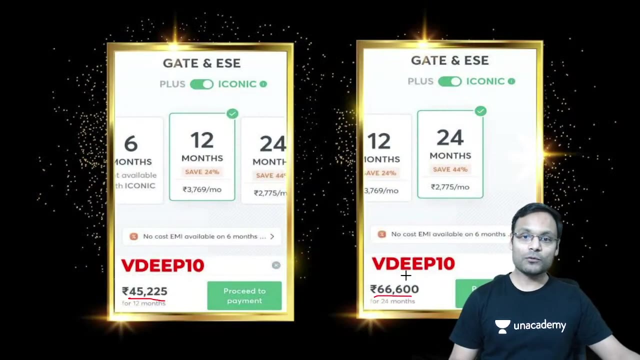 after that you will not have any new particular batch here. new batch will be starting, but not for evolve or for the ascend. batches means full length batches you will not be getting. look at these. these are the prices for 12 months, 18 months and 24 months for the gate and 12 months and 24 months for the iconic subscription. after the discount. 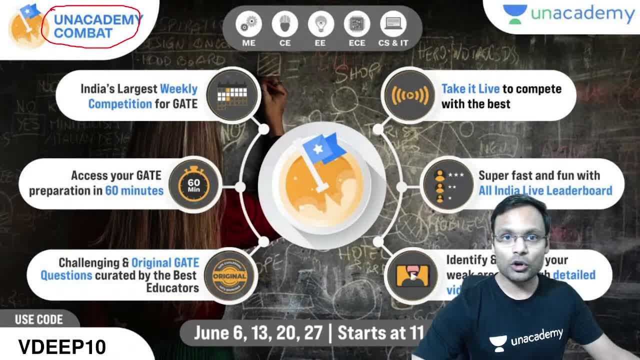 there is an opportunity for you to earn the scholarship for an academy plus. how write this scholarship test on academy combat which is going to be conducted on next Sunday, again 13th, 11 am. this will be the last nine days this particular, and can accommodate so that you can unlock this bomb. but 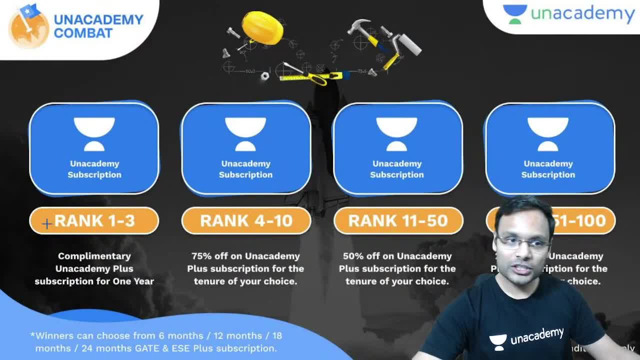 no, these costs with no any cost. this combat is a scholarship test. if you get ranked was between- this is calling shipped as we are- complementary subscription, you are going to get for your-plus- prescription. if you're convinced, looking back on back, you'll get 75%. 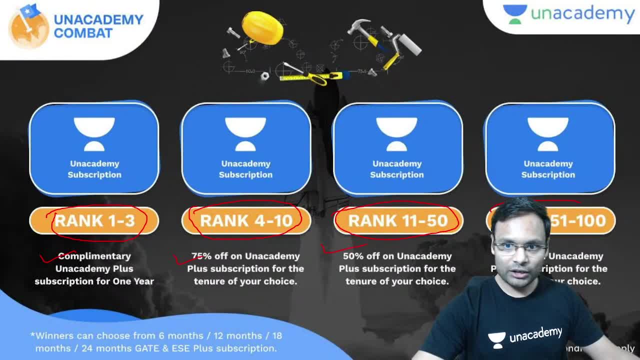 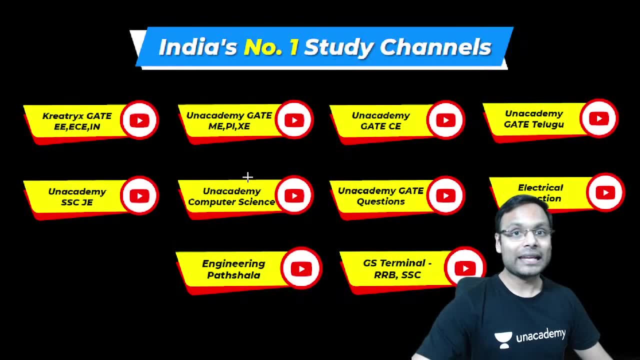 Does follow. if you're making, you see, even 250 person'd be started. if you're going to see you 1, 2, 1, 2, 125AAAA To get In this, this subscription of unacademy plus, if you are enjoying the sessions here, please support the.